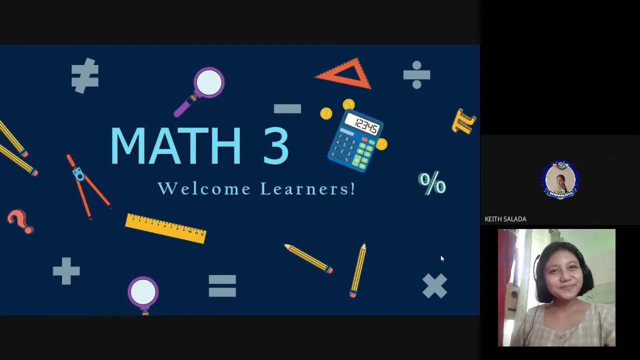 All right, so how are you, everyone? Are you good? Are you well? You can open your mics. Okay, good. 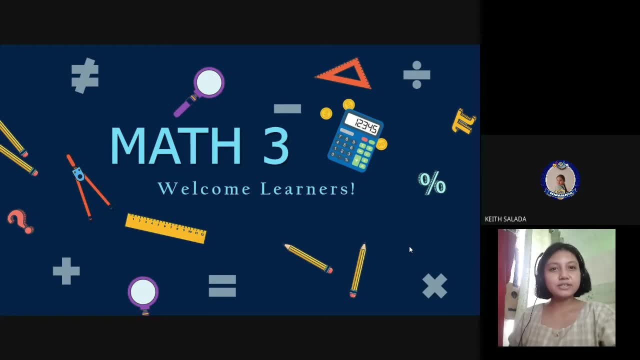 So I hope you are doing very well. So to everyone who has a stable... We're doing great, Miss. Yeah, so to everyone who has a stable internet connection, I encourage you to open your cams. 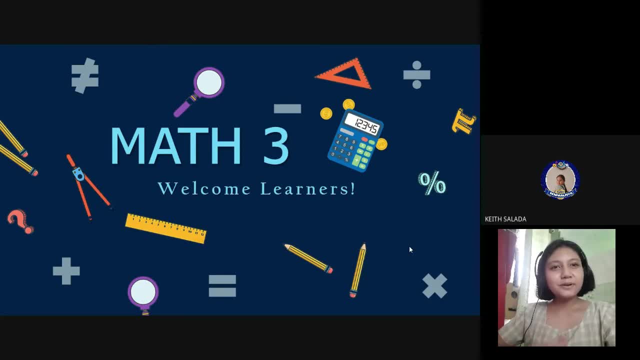 I really appreciate it if I see you, kay Murag, para makakita ko sa inyong beautiful faces. 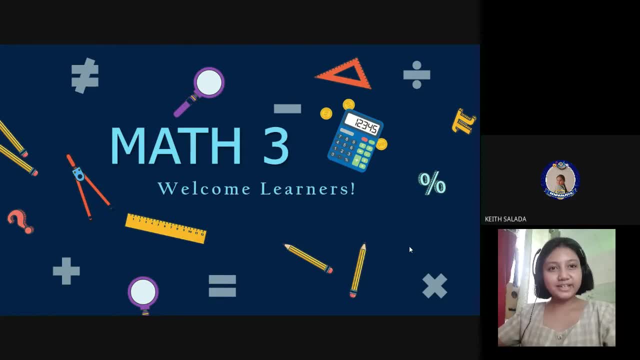 But if the signal isn't that stable enough, so it's fine. 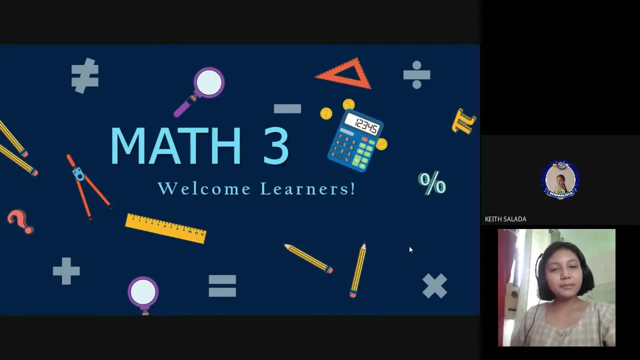 But I just want everyone to be attentive today, to cooperate. Is that clear? Is that clear? Is it okay? Yes, ma'am. Okay. So while I am checking your attendance here, I want everyone to open their mics and greet one another while I check if all of you are attending the class today. 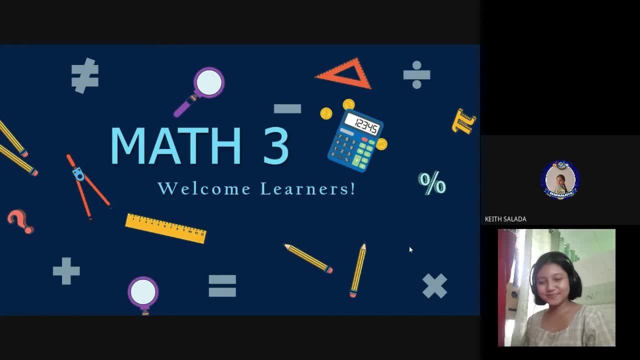 So open your mics, greet one another. 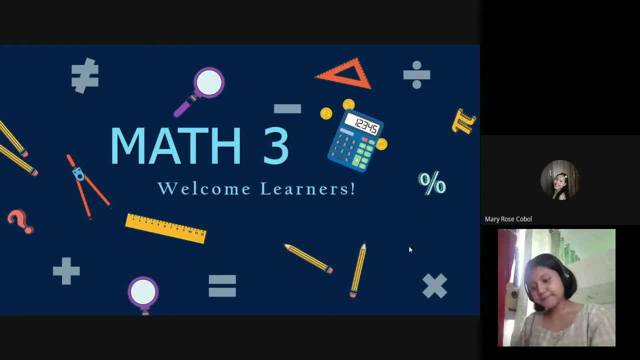 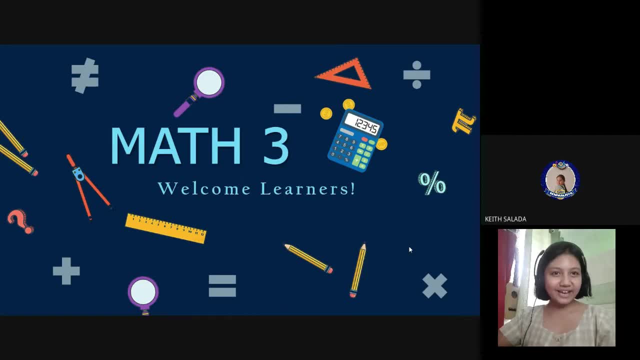 So I think everybody is here already. I am happy that you are all present today. I am Teacher Kay. And I am with Teacher Desiree. Teacher Des, say hi. Hi. Good morning. Good afternoon, students. Okay. So we will be your teachers in the math class today. So I hope that you are happy, just like us, that we're happy that you're here. So please be seated. 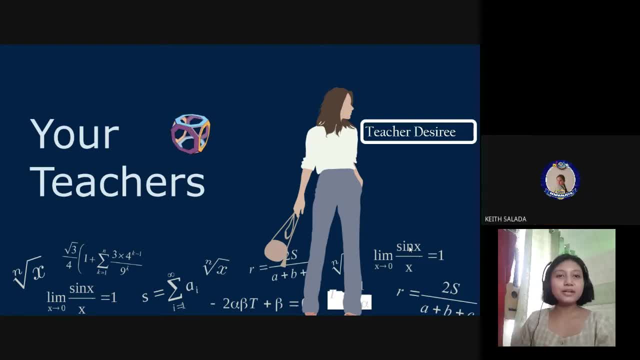 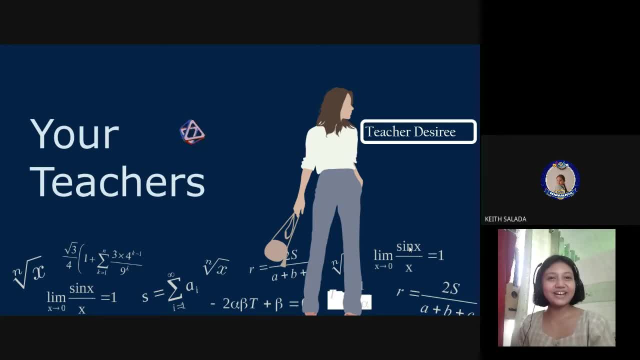 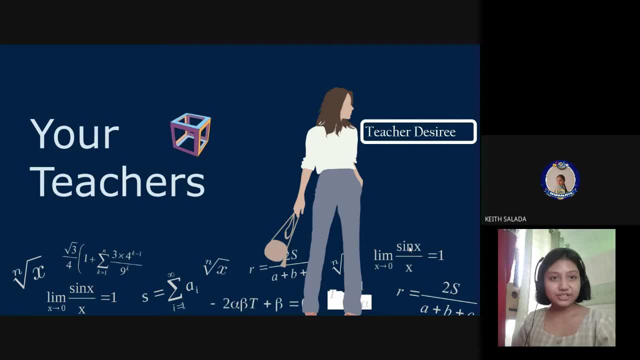 So, to finally start our class today, I want first to, you know, to stretch, to stretch your arms, stretch your necks, para maging active ta. O sige, stretching sa taon na, stretch your arms, then head rotation, ganoon. 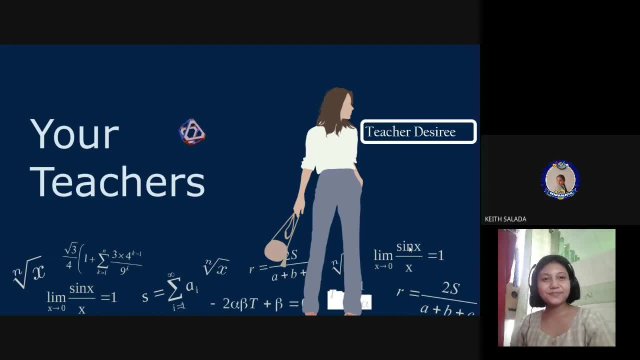 Okay, are you good? Are you good now? Yes, miss. 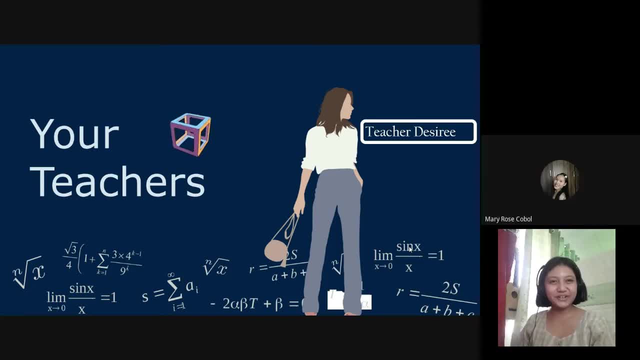 Yes, miss. Okay, very good. Thank you. Thank you for the response. 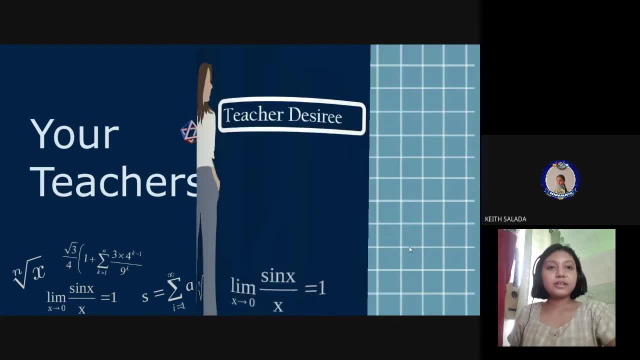 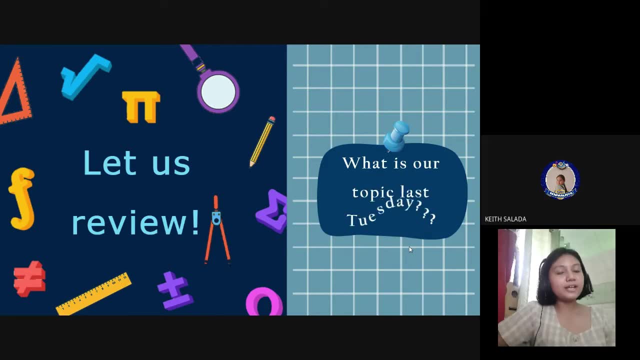 So now, so to start, we'll just review what did we tackle last Tuesday? What did we learn last Tuesday? 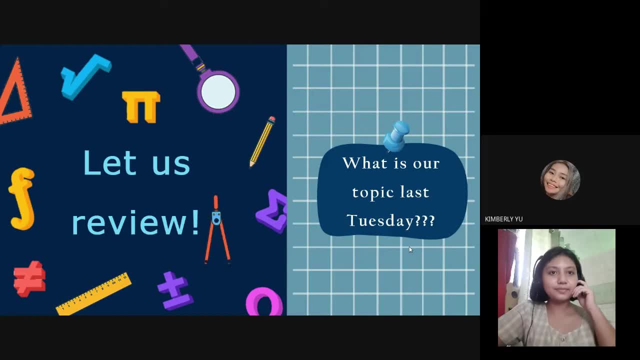 Anyone? Me, miss. 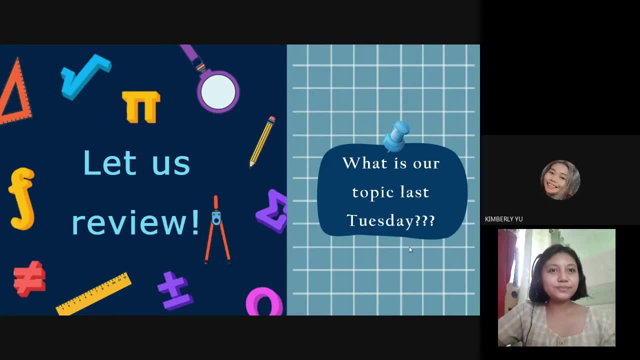 Okay, Kim, go ahead. It's all about addition. 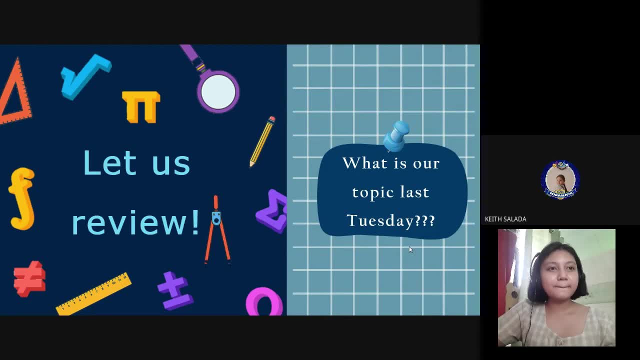 Addition, miss. Okay, very good. Good. Very good. It's all about addition. So up to how many digits? How many digits did we sum last Tuesday? 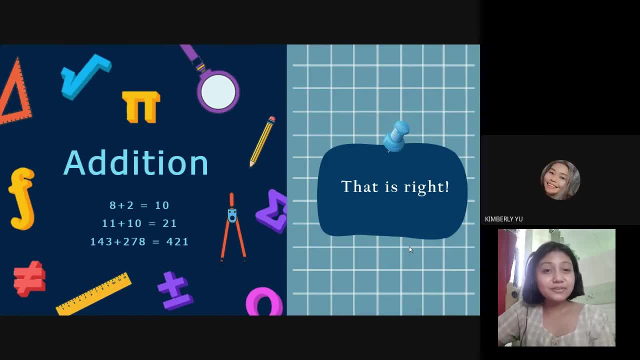 Kim, are you there? Yes, miss. Up to how many digits did we sum? Three. 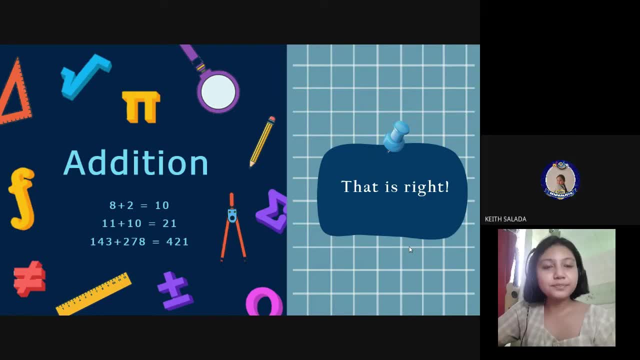 Okay, very good. Three. Three digits. Okay. 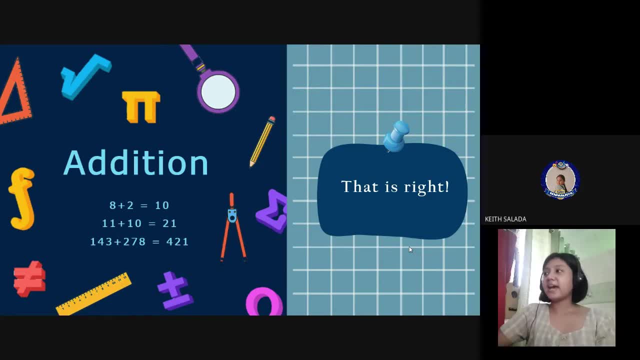 In the screen, we have an example of addition, right? Equation. 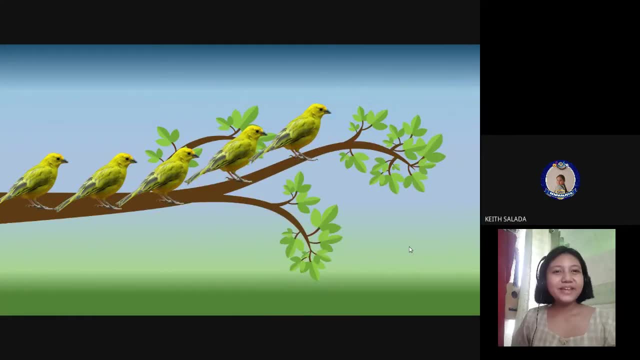 So now, so now, let's sing a song first, an action song. Do you know the song? Chika-ding, chika-ding, naglupad-lupad. Okay. 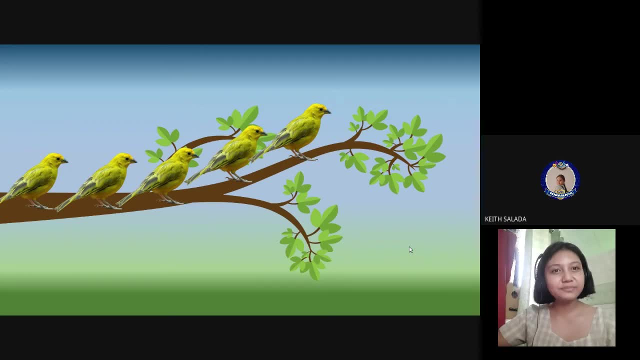 So let's learn this song. So we have, I have here pilamangkabuk birds. Pilamangkabuk chika-ding nasa screen. Five, miss. Five. Five. Very good, Shane. So we have five chika-dings here on the branch, right? 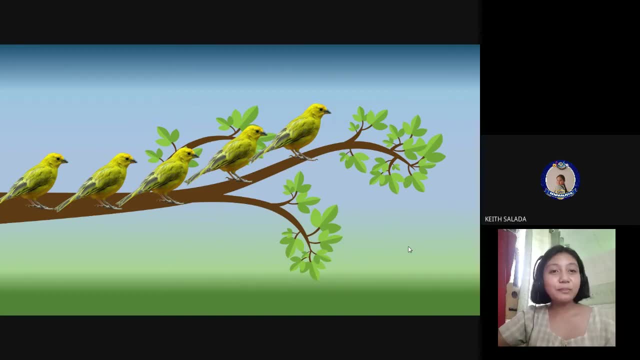 So sa song, chika-ding, chika-ding, naglupad-lupad. Diba mo fly mo ng birds, right? Okay. 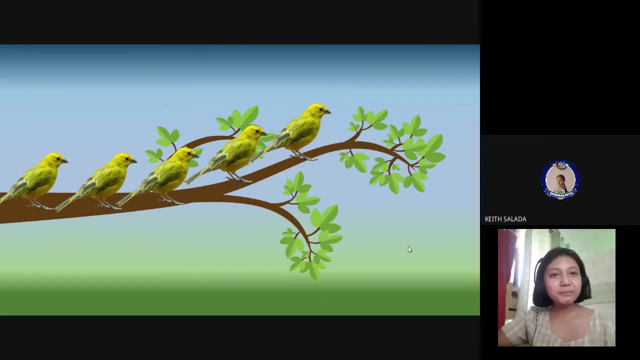 So we'll sing that song. Are you ready? So follow with me na lang ha while naka-unmute mo. But I want you to count with me. Okay. Okay, thank you. Okay, miss. Ready? Chika-ding. Ready? Sing. Chika-ding, chika-ding, naglupad-lupad. 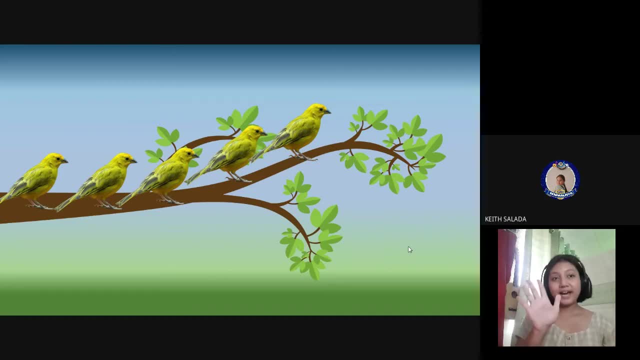 Chika-ding, chika-ding, naglupad-lupad. May lima ka chika-ding ning batok sa sanga. Nilupad ang isa. Pilamang sila. Upat na lang sila. Upat na lang sila. Chika-ding, chika-ding, naglupad-lupad. Chika-ding, chika-ding, naglupad-lupad. May upat ka chika-ding ning batok sa sanga. Nilupad ang isa. Pilamang. Three. 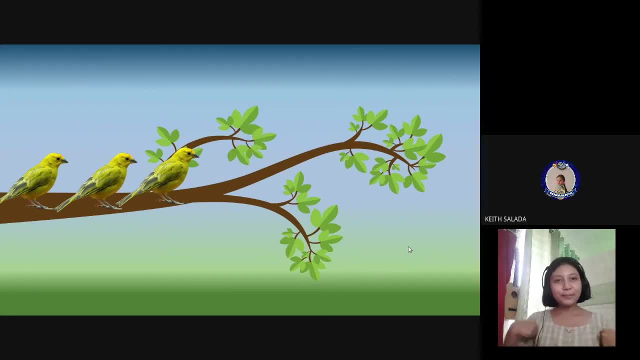 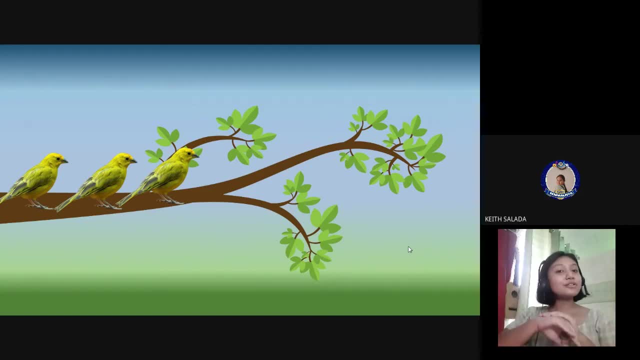 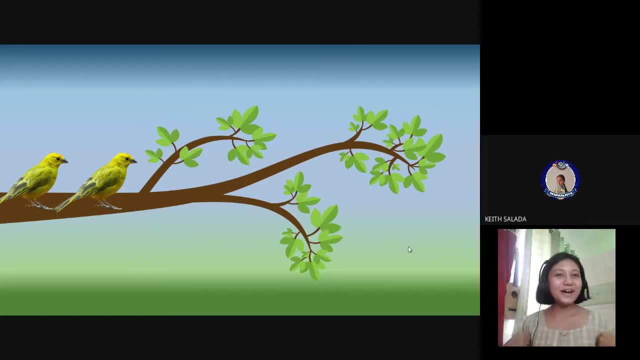 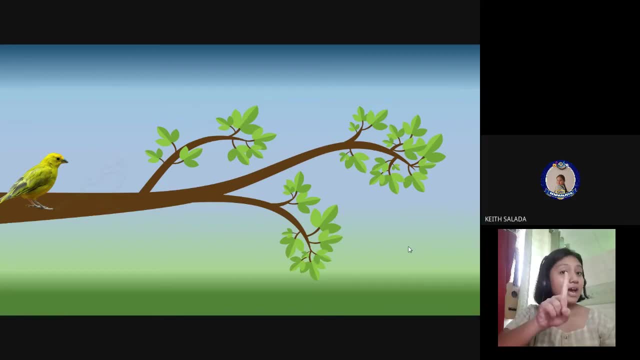 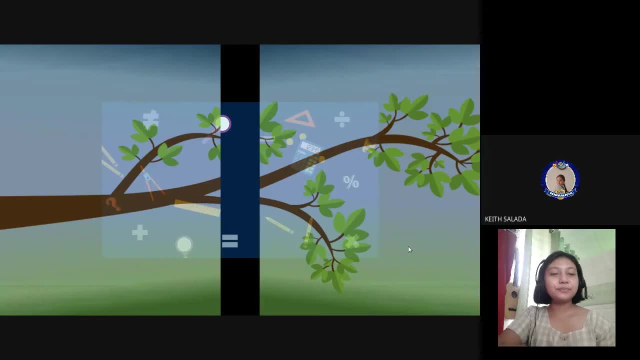 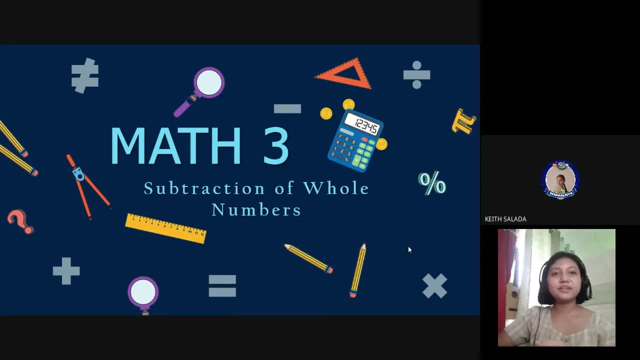 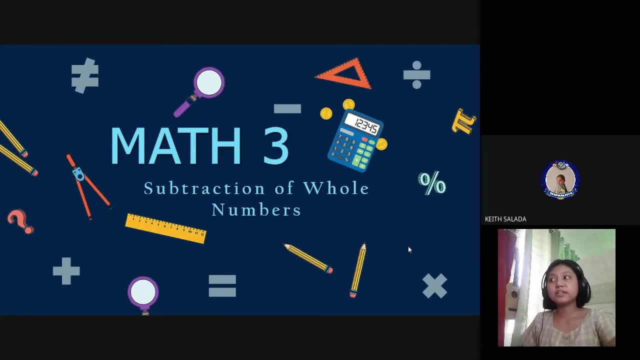 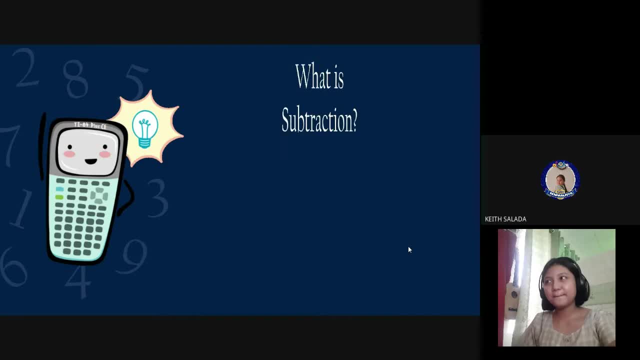 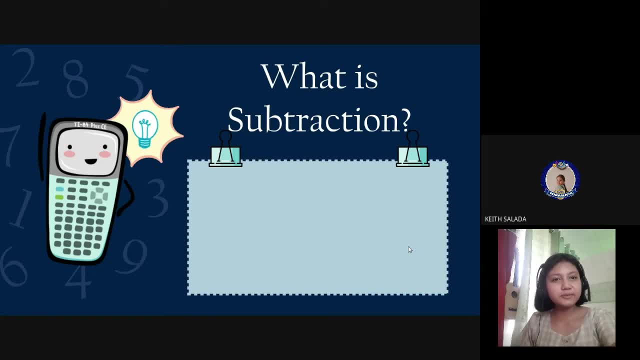 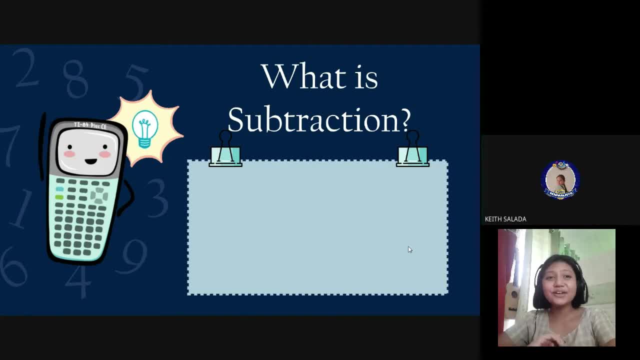 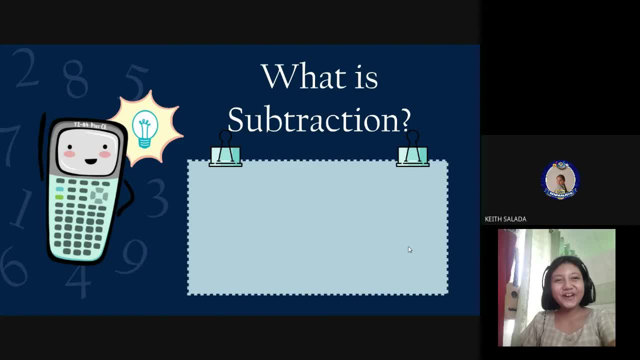 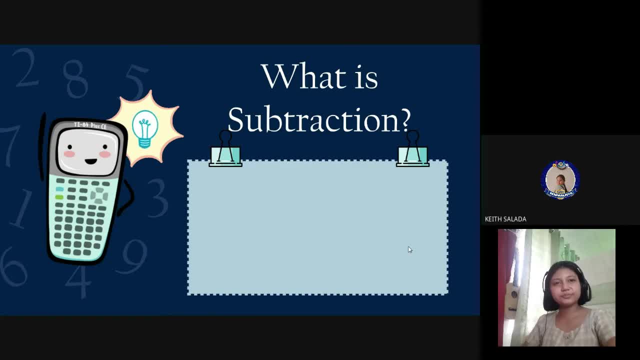 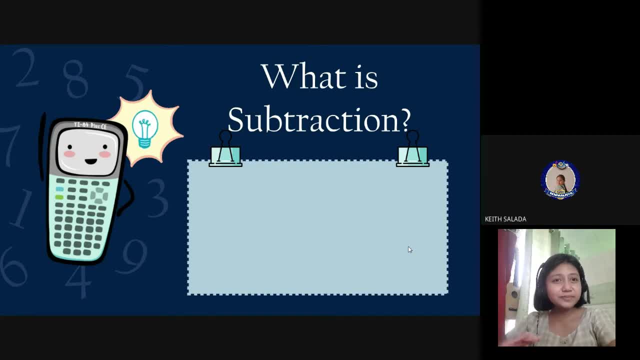 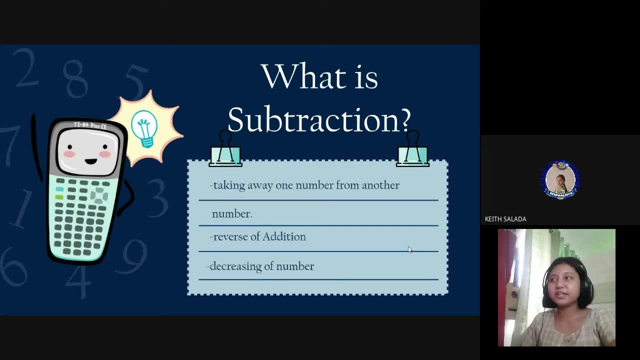 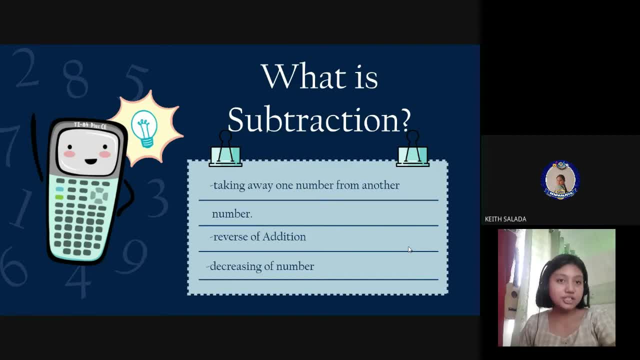 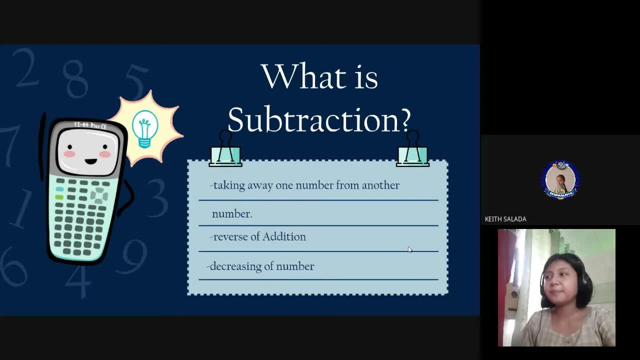 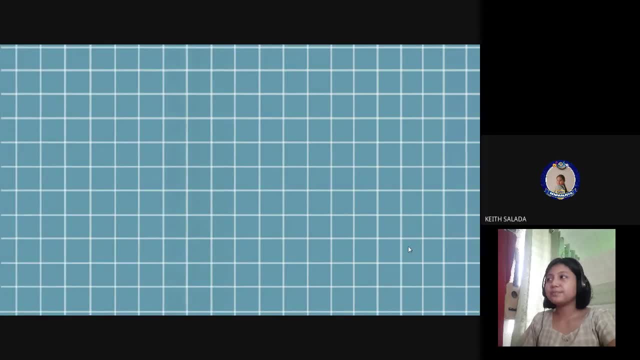 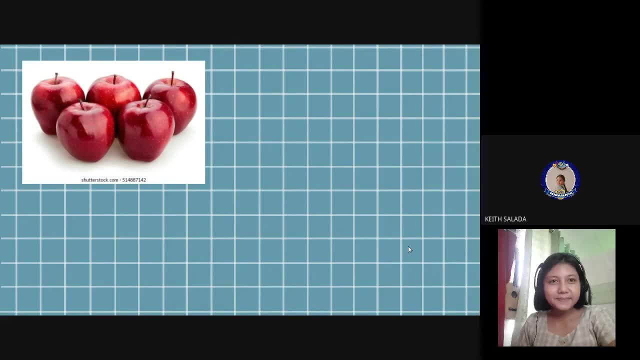 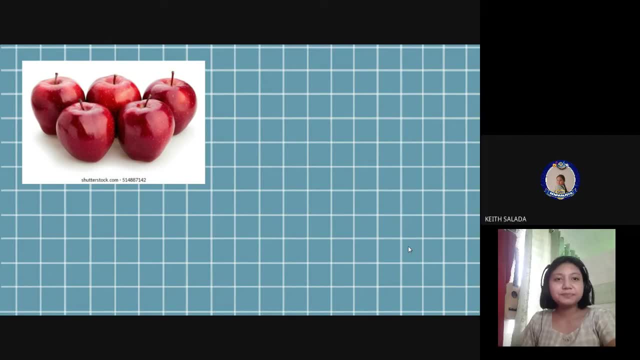 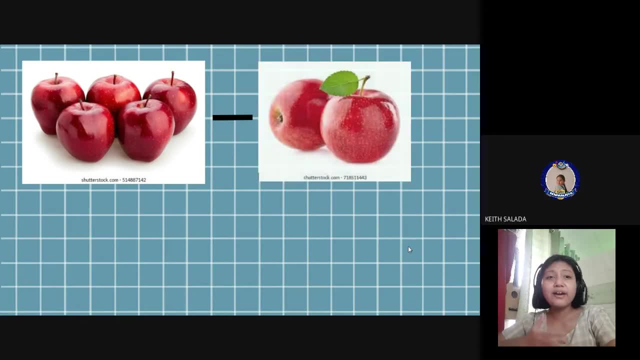 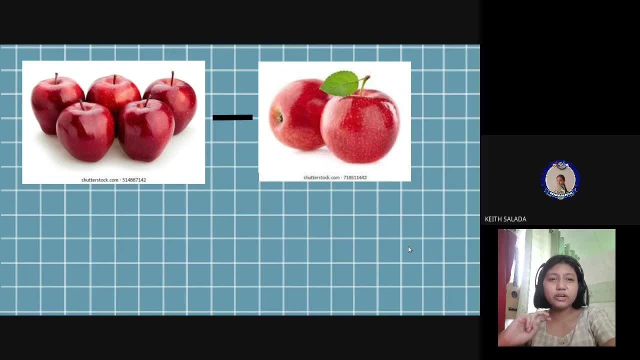 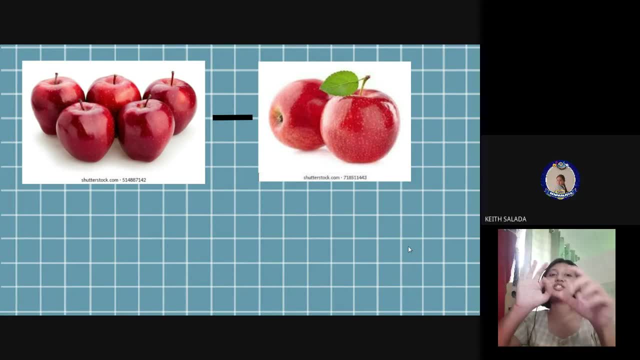 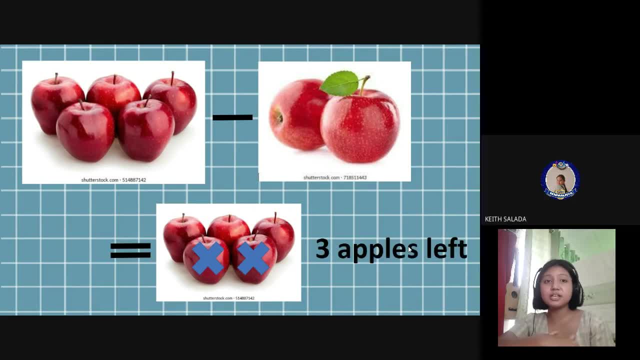 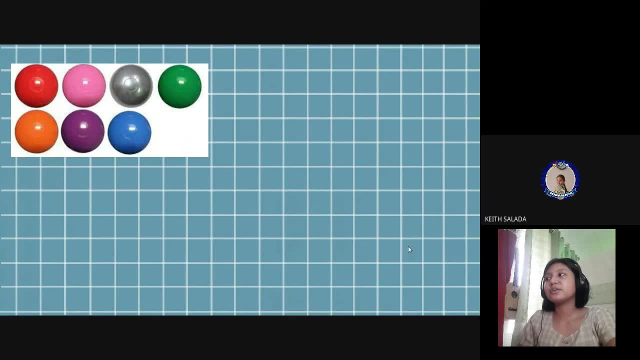 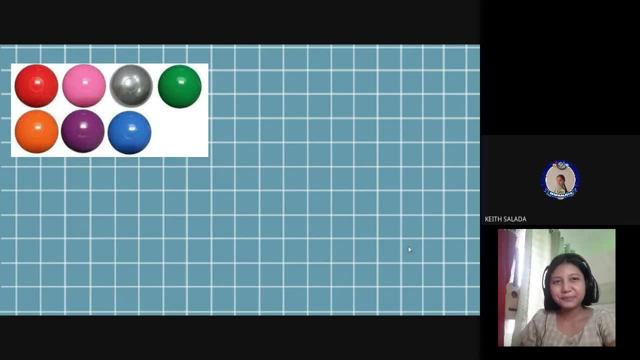 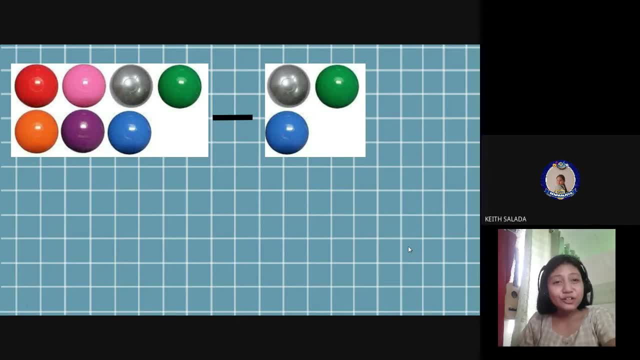 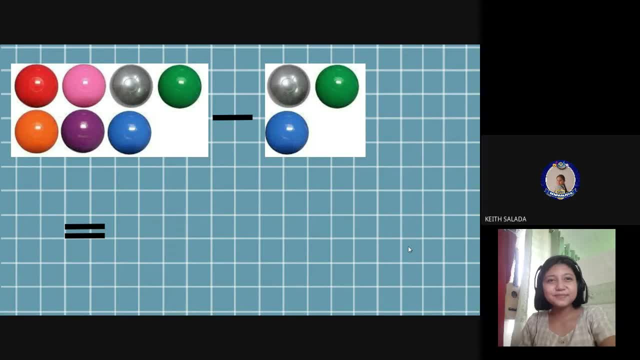 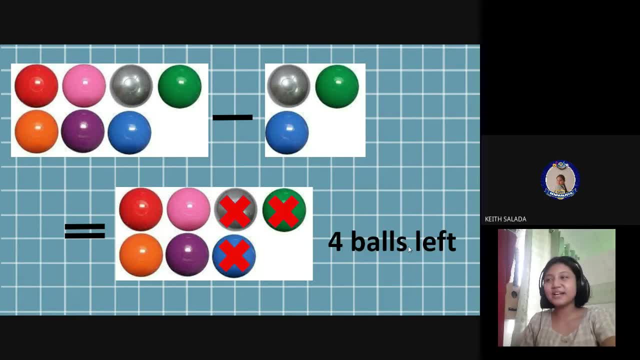 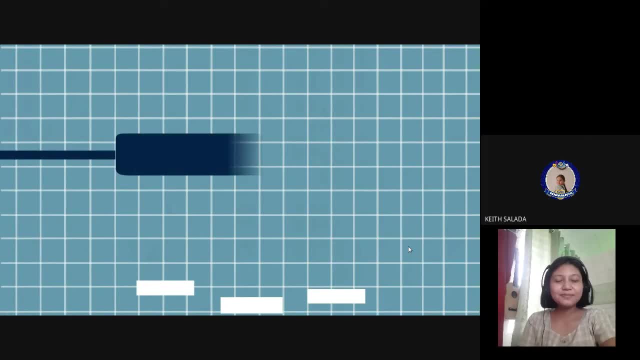 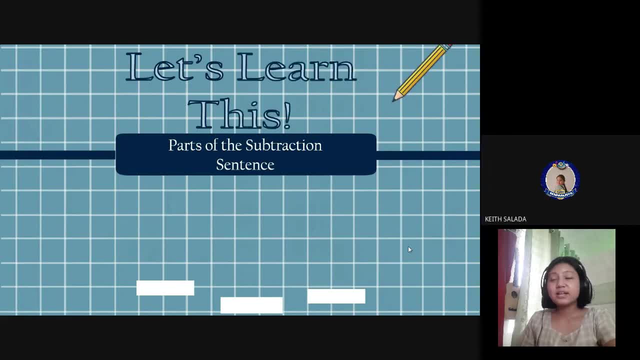 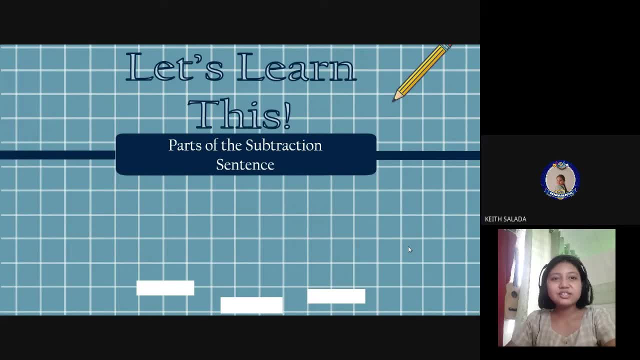 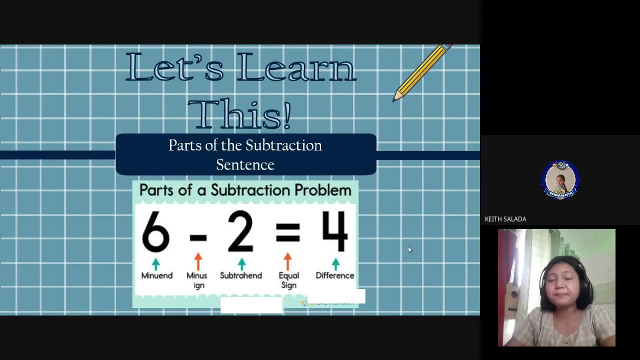 So we'll learn about the parts of the subtraction sentence What are the parts of the subtraction sentence? If the addition is an addition sentence, it can be a subtraction sentence What are the parts? So here, I have an equation 6 minus 2 is equal to 4 So 6, what is this? 4 So 6 is called, in the subtraction sentence, called minuend Okay, repeat after me What is the name of this? Minuend Minuend, okay, minuend 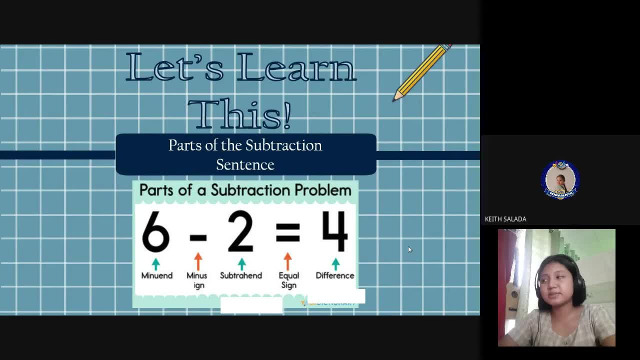 And then, here's the minus sign This represents the subtraction The minus sign Okay, the 2, this is called the subtrahend What is it called here in number 2? Subtrahend Okay, subtrahend, very good So we have the minuend, the minus sign Then, next to the minus sign is The subtrahend Followed by the equal sign The subtrahend here is Pilakabuok imong kuhaon 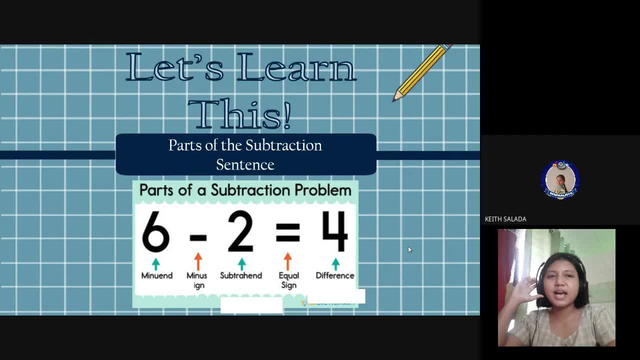 Okay, so Since the subtrahend here is 2 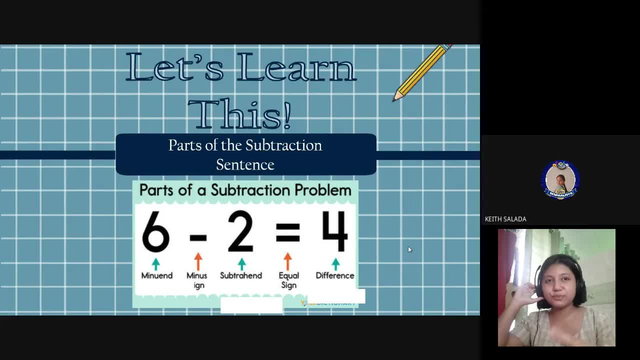 So 2 is the minus, right? 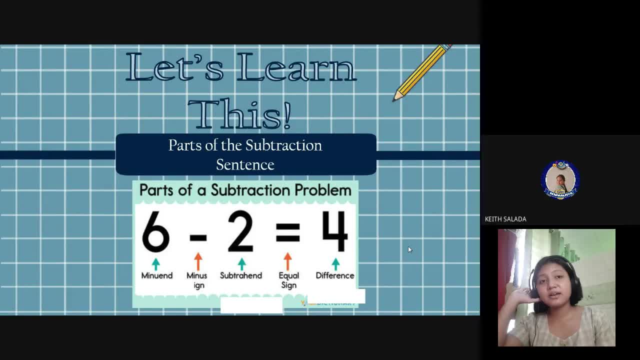 So equals Then, the difference in the given Is called difference What is it called? 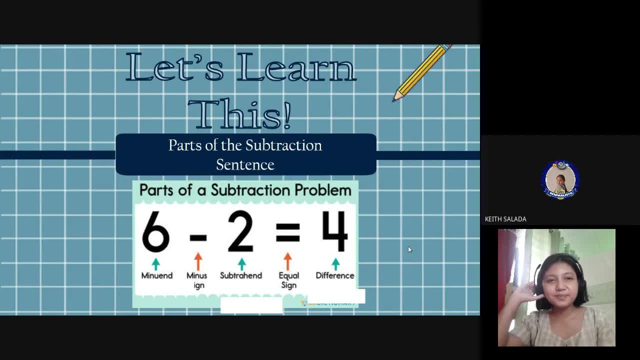 What is it called again? Difference 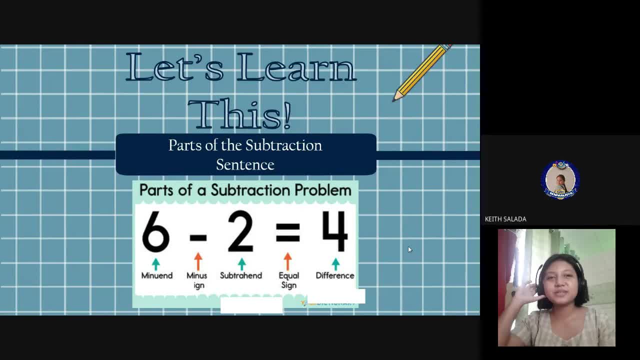 Okay, difference So this is called the answer in the subtraction Get it? The minuend, minus sign, subtrahend, equal sign And then, followed by the difference 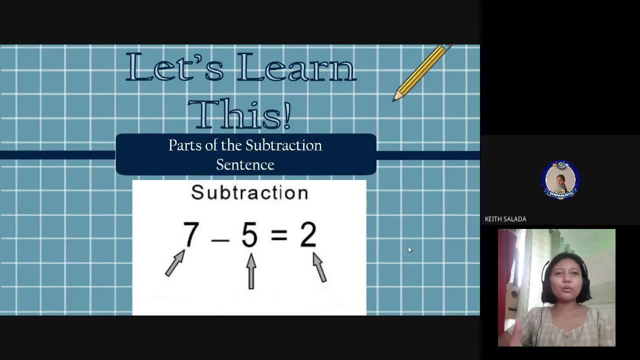 Okay, so now, so that I can see more Or I can get your answer 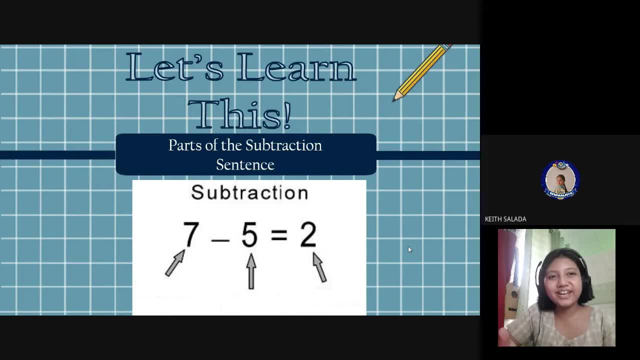 I will ask Jasper Jasper J Jasper J Okay, nice, the name 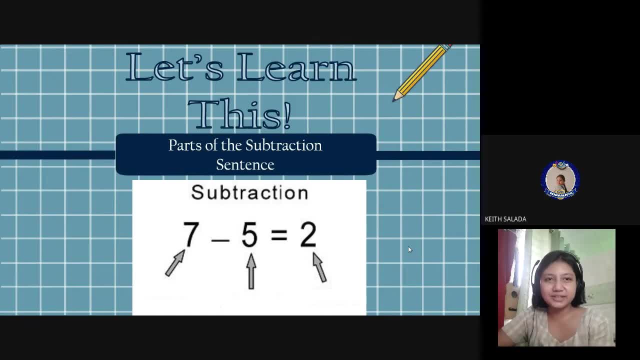 Jasper J What is the name of the seventh? 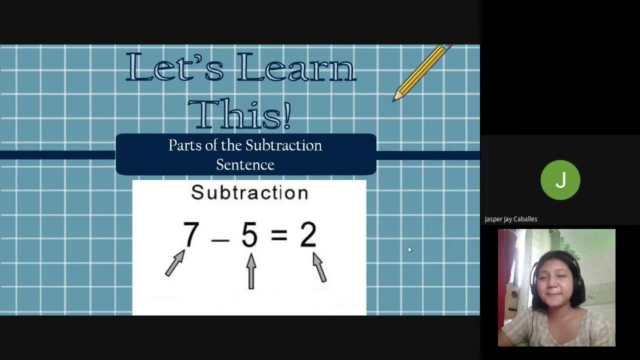 What is the part? Minuend Very good Minuend And then, the fifth, Jasper? Subtrahend 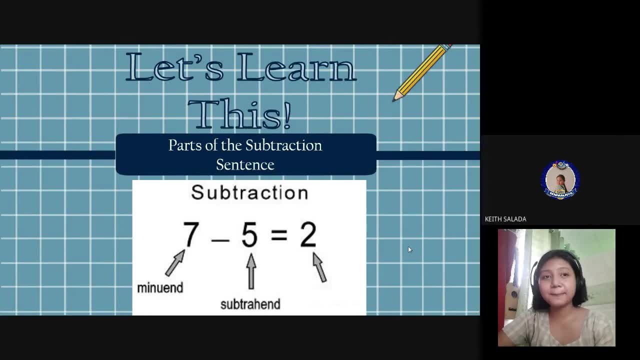 Very good, subtrahend, okay Then, I will ask Kim What is the name of the number 2? 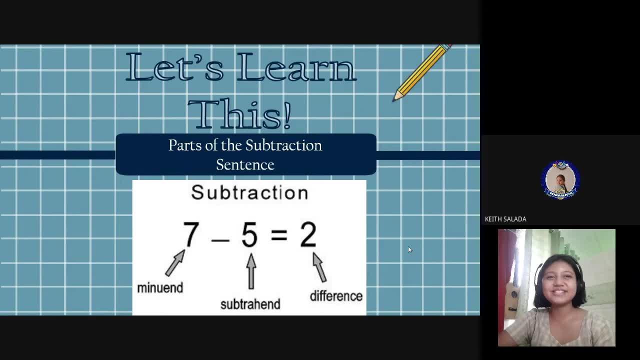 Difference Okay, difference Okay, so 7 minus 5 What is 7? 5 is equal to 2 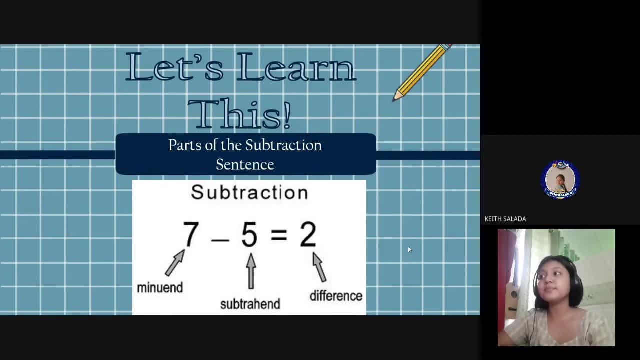 So the difference is 2 Okay, good, right? 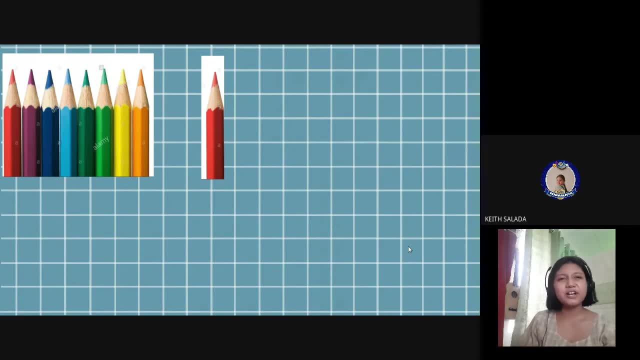 Okay, so to further visualize this So that you can see more So that you can see more pictures So that you can see more of this So I have here 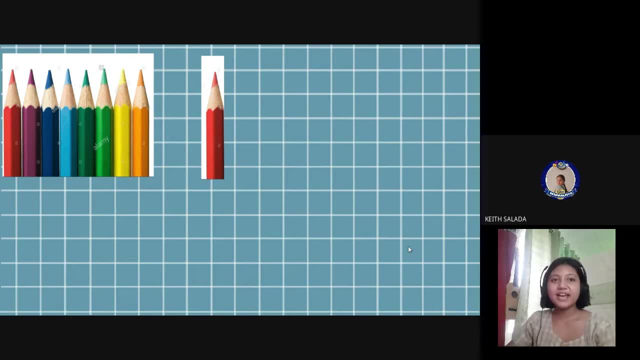 1, 2, 3, 4, 5, 6, 7, 8 8 colored pencils And then 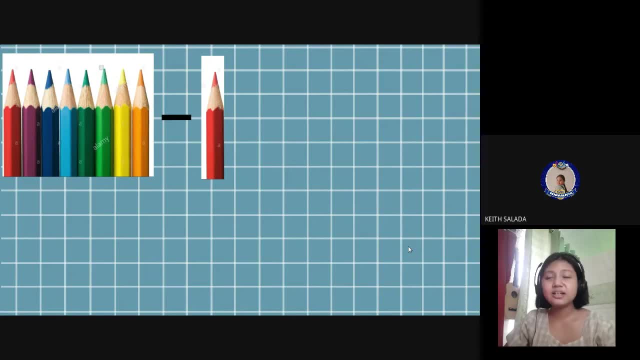 What will I get? What will I get? 1 So 8 minus 1 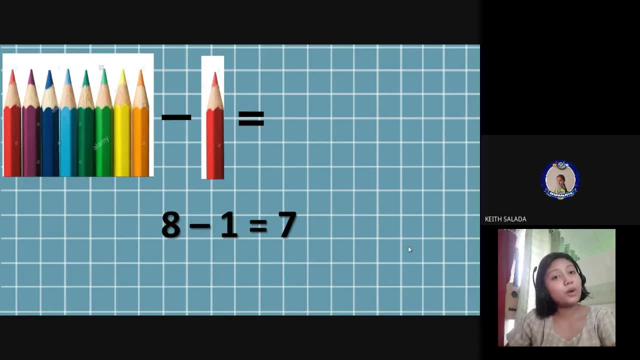 So the subtraction sentence will be this 8 minus 1 is equal to 7 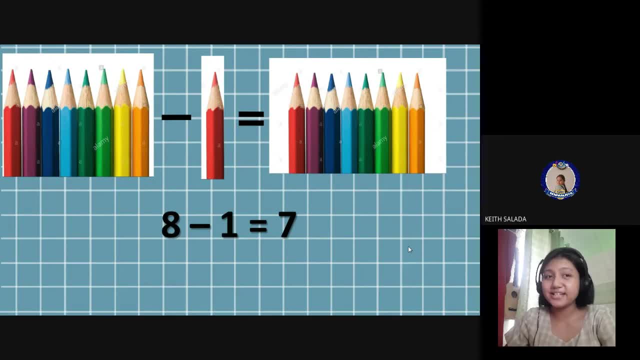 Okay, so this is the subtraction sentence Did you get it? So far? Did I pass? Yes, Miss 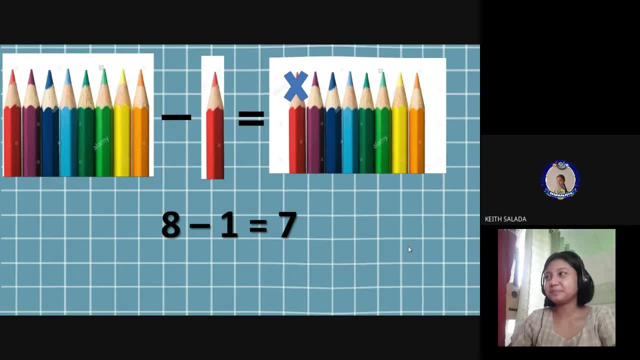 Okay Did I pass? Okay Let's move on 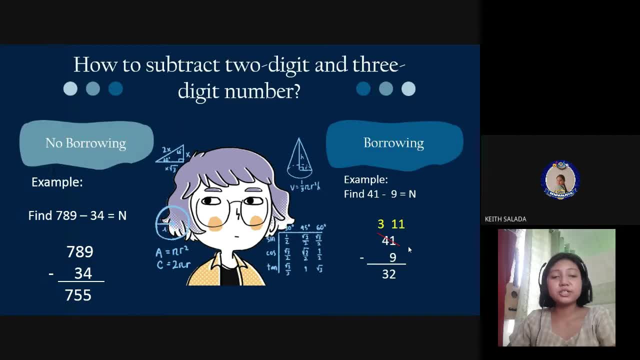 Okay, so Since we already know the subtraction sentence The parts of the subtraction sentence How to subtract 1 digit So now let's move forward to How to subtract 2 digit and 3 digit number So there are 2 rules In subtracting 2 digit and 3 digit The no borrowing and the borrowing So in no borrowing, I have examples here So you have the equation of 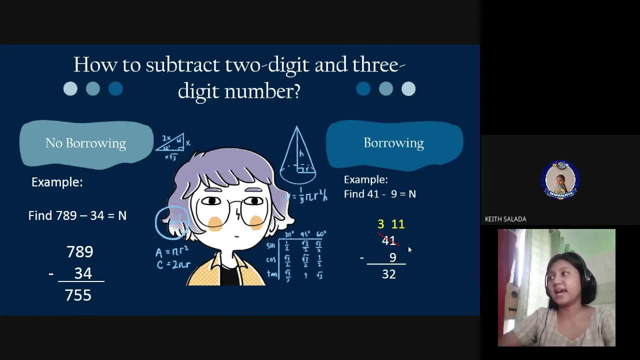 Find 789 minus 34 is equal to n So n here represents the difference Or the answer is different Right? 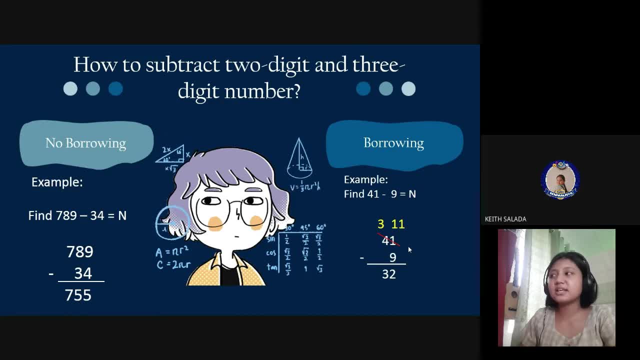 So where is the place value of 1 here in 789? Where is 1 here? Okay Okay, Kim 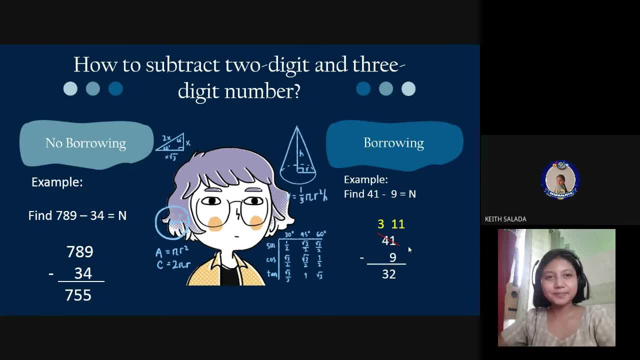 Where is the place value of 1 here in 789? Right here, Miss Okay, very good Right here, 9 And then, Shane Is Shane around? Okay 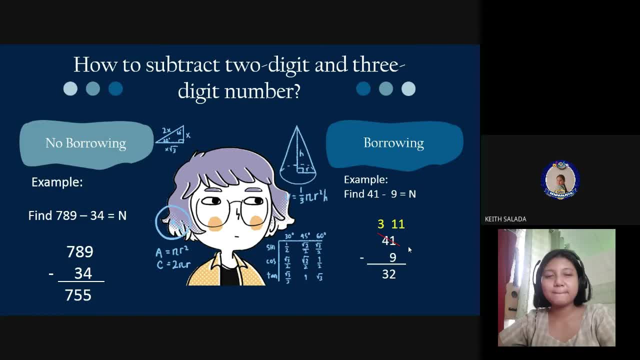 Shane, where is the place value of 1 here in 34? 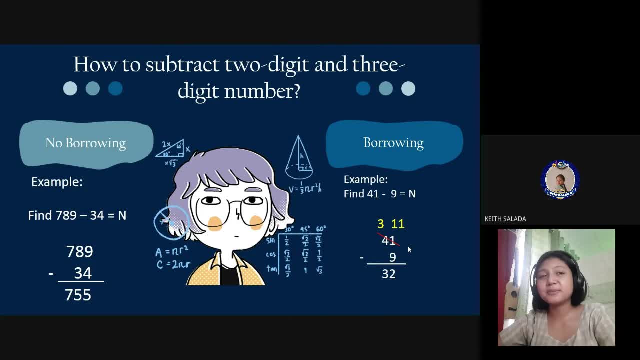 4, Miss Okay, 4 So to For us to understand So we will align The ones that are in the place value of 1 So 789 minus 34 So let's align 9 and 4 And then the 10th digit of 789 is 8 And then the 10th digit of 34 is 3 Right? So let's align them So here, it will be a circle So 9 minus 4 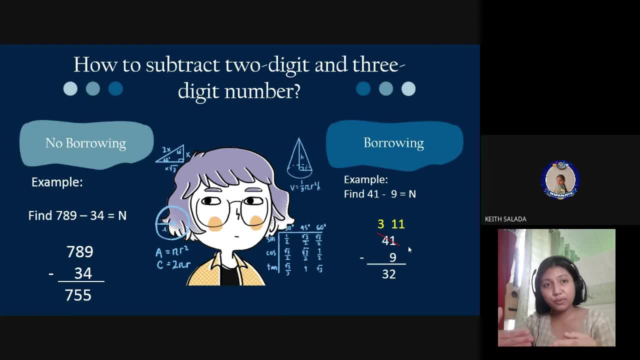 Once after you align it You subtract it So 9 minus 4 is equal to The number of Let's see here Mary Rose What is the number of 9 minus 4? 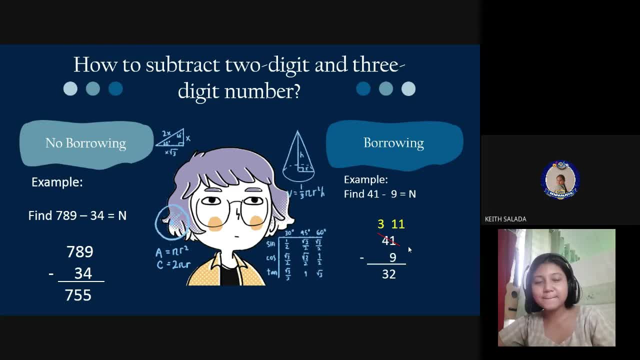 Is Mary Rose around? Okay, so Mary Rose is silent Okay Nothing? Okay, may I call Sorry, Miss Okay 5 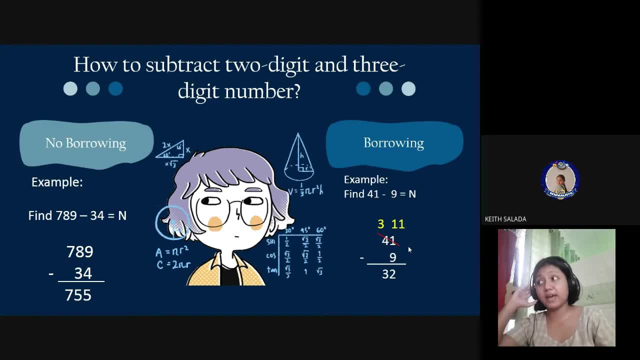 5, very good 9 minus 4 is equal to 5 And then Mary Rose, let me ask you again 8 minus 3 What is the answer? 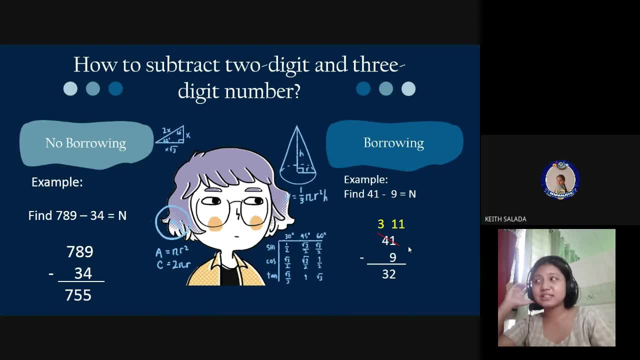 Is it equals to 5 8 minus 3 5 5 Yes 5 So since there is no 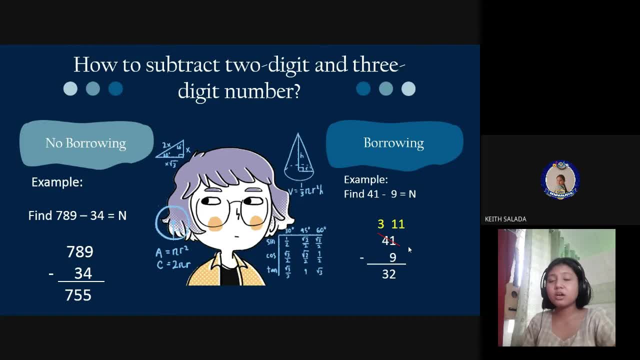 There is no place value of 100 in 34 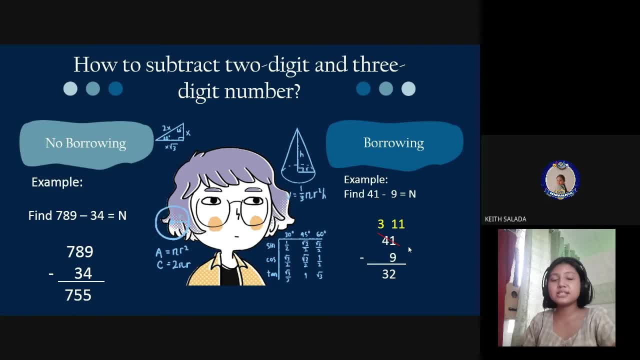 So there is no one that is aligned with 789 Or 34 in the 100th place So let's bring down this Let's bring down this 7 So the difference in 789 minus 34 Is equal to 755 Okay, did you get it so far? Okay 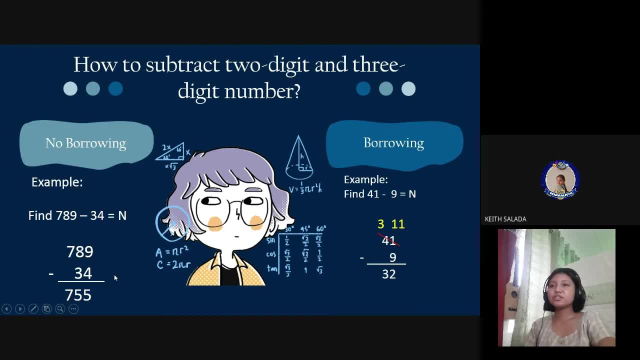 So now let's proceed to borrowing So I have here an example of 41 minus 9 is equal to n 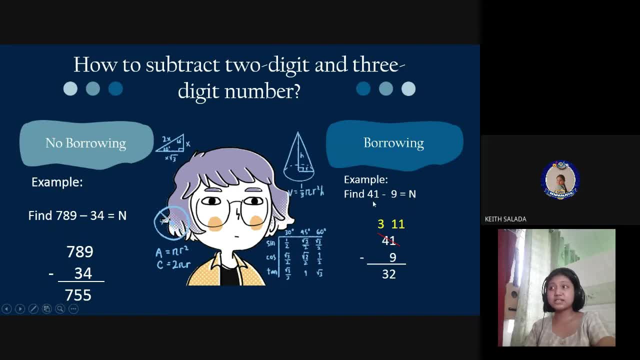 Again, let's look at the answer In 41 minus 9 Okay, so just like what we did a while ago 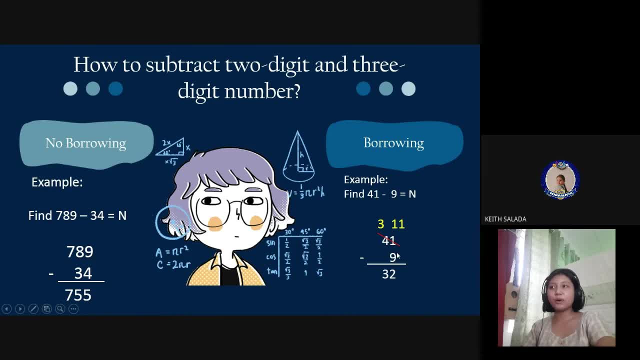 Let's align the ones The ones that are placed Then the tens Then the hundreds Right? So for 41 Let's align it with 9 That is in the ones Okay Ones placed Okay, so 1 minus 9 Which one is more expensive? Shane, which one is more expensive? 1 or 9? 9, Miss Okay, 9, right? Where is it? 9, Miss 1 minus 9? There, there How about 9? 9 or 9 plus 7? 9 Okay, so So far 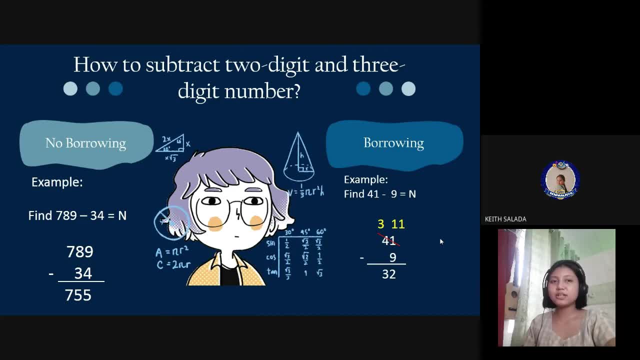 We are using the borrowed number The borrowed number The number that comes in first In the place value Of 1 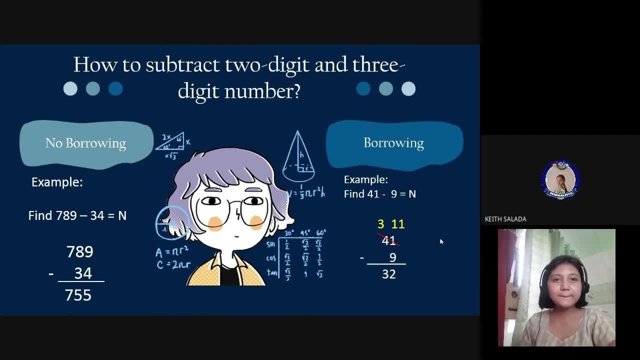 Okay Which number came in first In 1? Shane 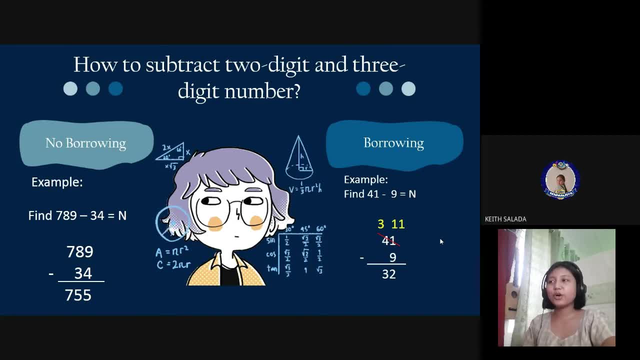 4, Miss Okay 4 Very good 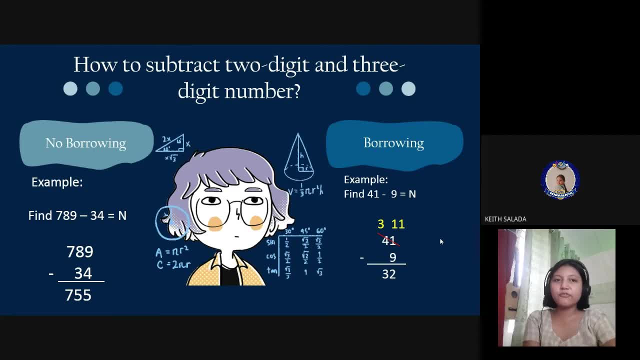 So 4 Since We got kuwan ang 4. So, pwede na to siya ma-crush outan. Pwede na to siya mahugman ang number. 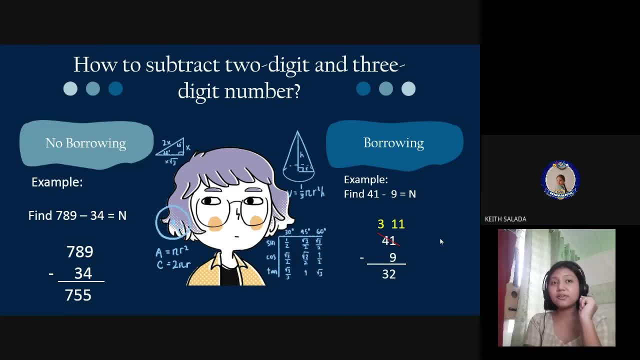 So, crush outan na tong 4. Mahay mo na lang siyang og 3. 3. Crush out na to. 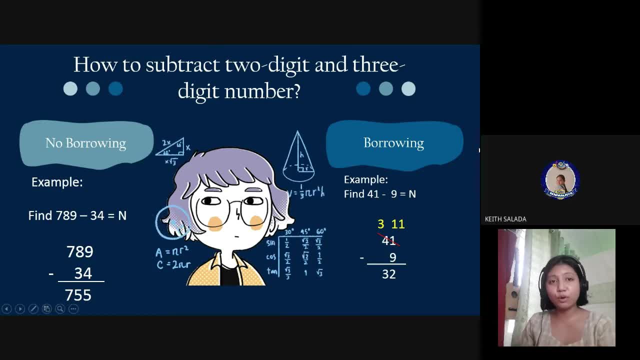 Mahay mo siyang 3. And then, ang gihulam na tong number sa 4, iba 1. Hulam tag 1. 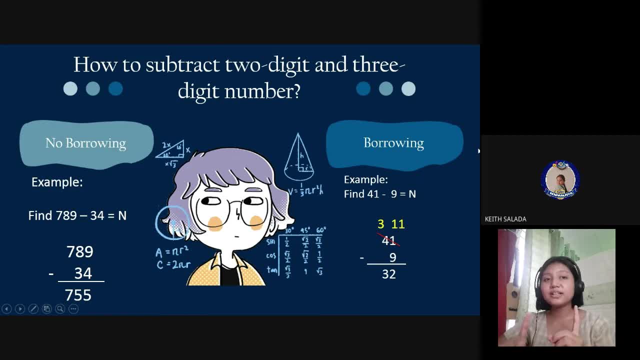 So, itapad na to sa 1. 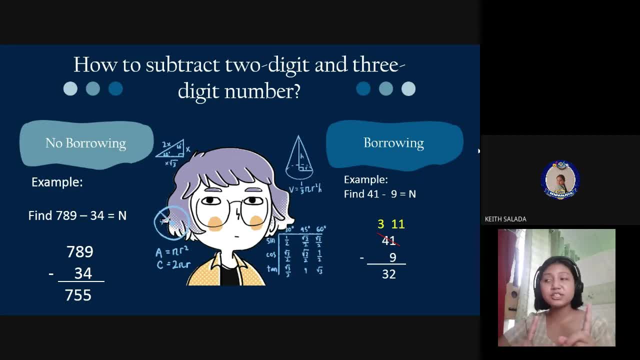 Nga na sa 1's place. Itapad na to siya. Mahay mo na siyang 11 over 9. So, possible na ba? Very good. So, possible na ba nga maka-minus? Yes, miss. Yes, thank you. 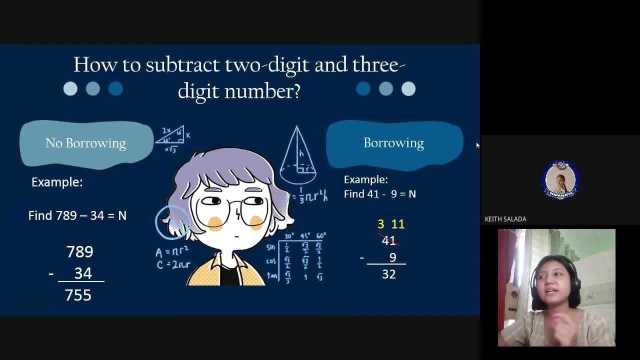 So, 11 minus 9, possible na nga maka-minus. So, pila ang answer. 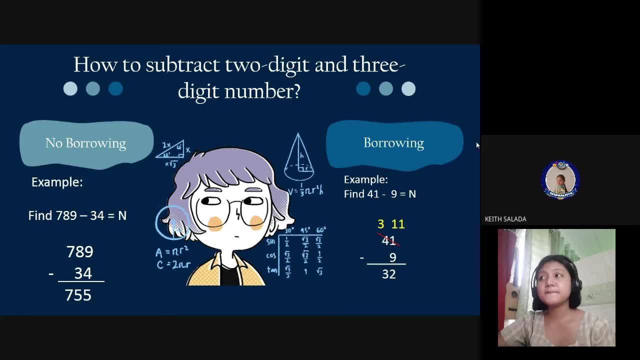 11 minus 9 is equal to? 2. 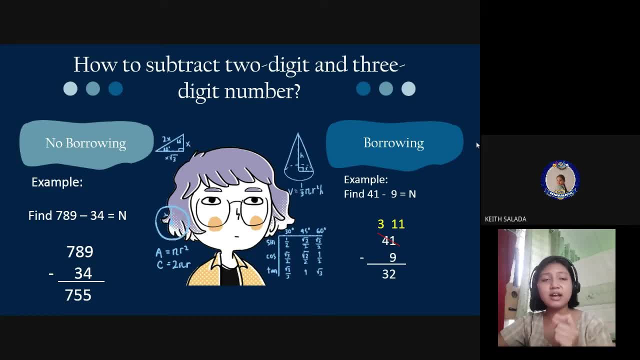 It's equal to 2. So, since wala may 10's place dito sa wala may 10's place dito sa subtrahend nga 9, so, i-bring daw na tayon si 3. 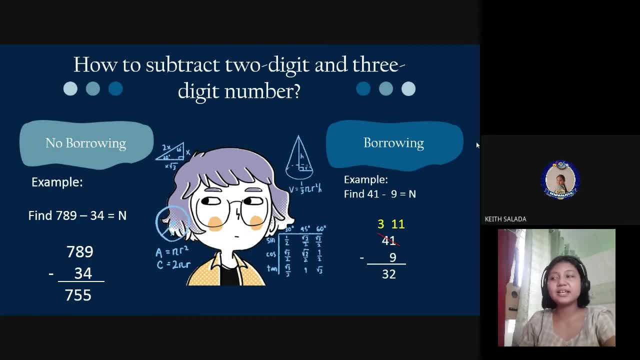 So, ang difference di ay sa 41 minus 9 kay 32. 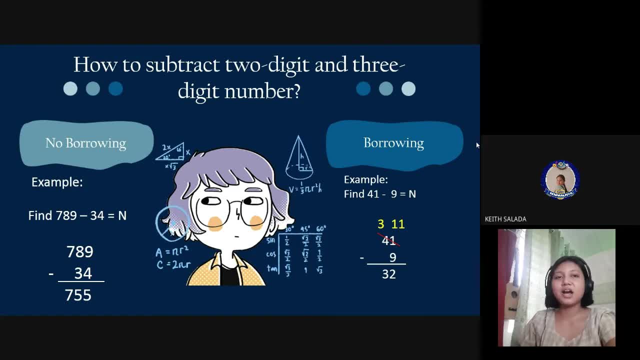 Okay, gets ra? So, maunay siya pag-use sa borrowing. Okay, gets so far? Okay, so now, let's proceed. Okay. 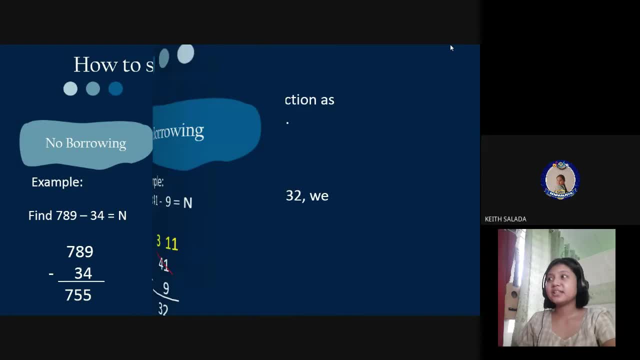 So, let's proceed. So, did you know that pretty much, 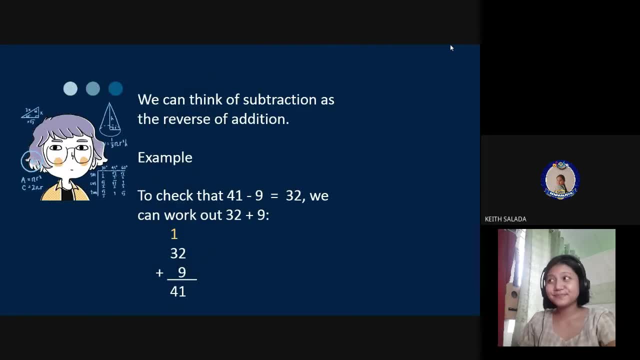 pwede na ito ma-check ang atong answer by using the addition. So, as I said a while ago, 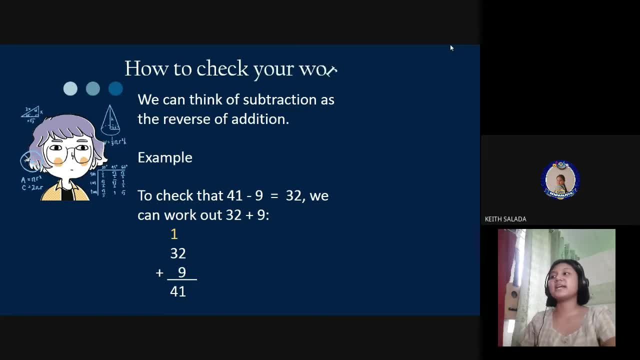 ang subtraction is the reverse of the addition. 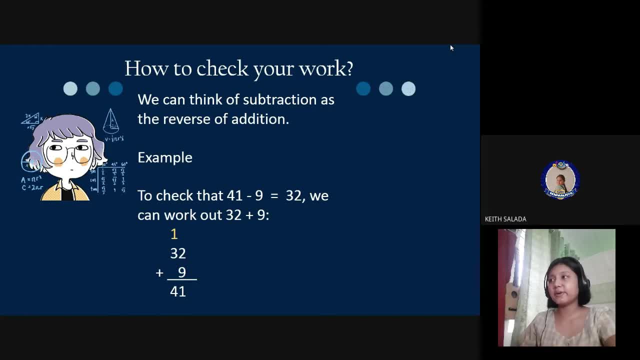 So, pwede na ito ma-check ang atong answer, ang difference 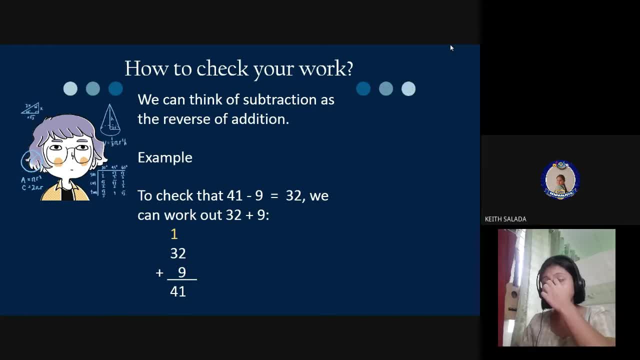 by using the addition. So, saan man teacher? Okay, so, 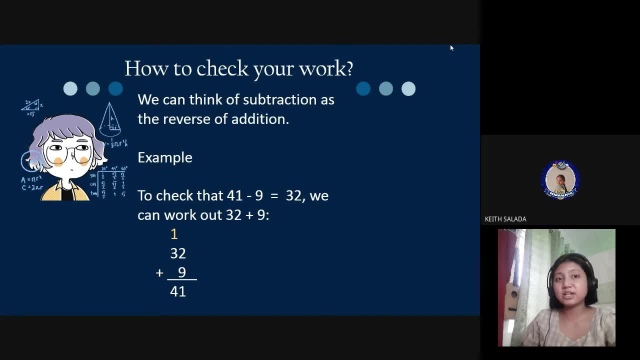 a while ago, we subtract 41 minus 9, diba? Ang answer is 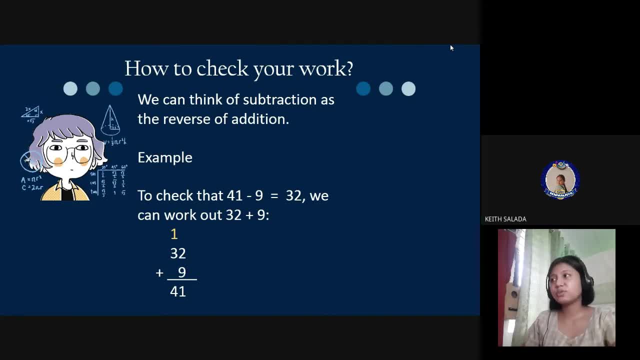 32, right? So, to check, kung sakto ang 32, we will use the number 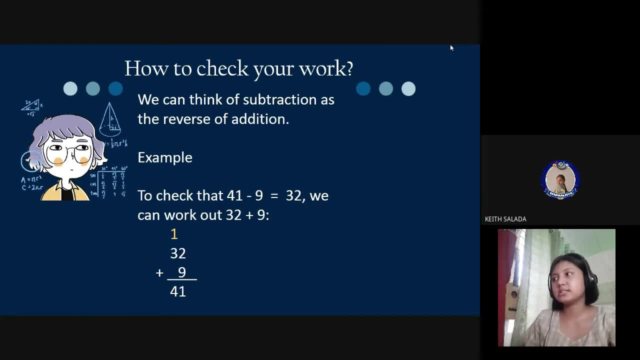 32 to add the subtrahend nga 9. Okay, so 32 plus 9 9 plus 2 is equal to 1, then 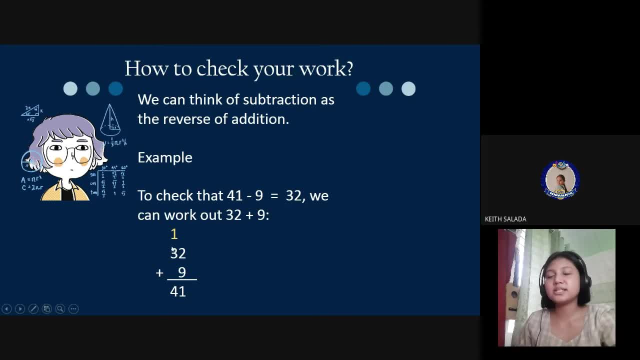 sa iba ba, 1, then 3 plus 1 kay 4, right? So, 32 plus 9 is equal to 41. Okay, so number 41 diba sa equation na ito sa first? Okay, naa siya sa very good. 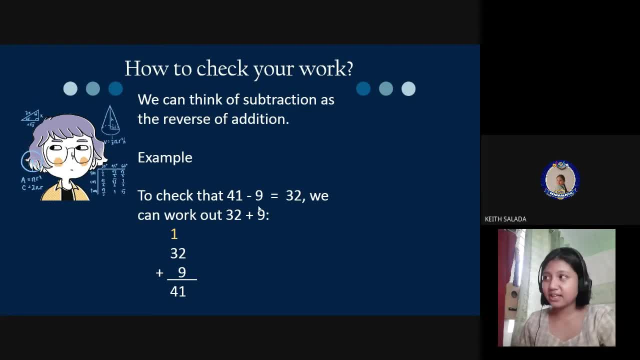 Naa siya sa minuend, right? So, this will check if sakto bagod ang answer nato nga, 32. 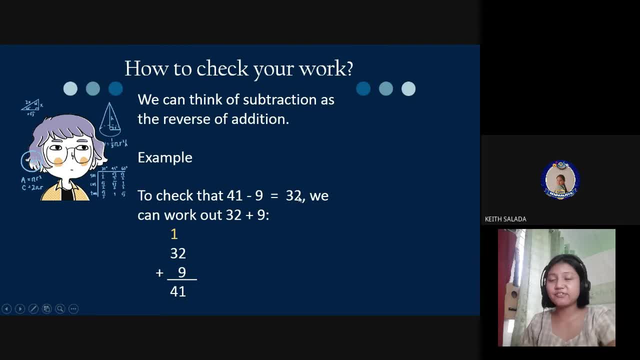 Okay, so, i-add ang difference and then ang subtrahend, and then ang mugawas kay ang minuend. 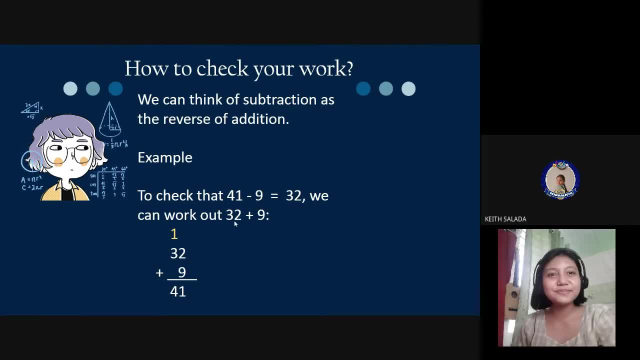 Okay, gets ra? So far? Gets ra? Kaya ra? Yes, teacher. Okay, thank you. Thank you, Kim. So, now, 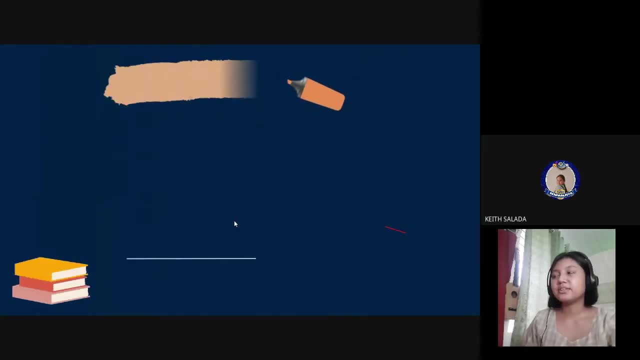 I will give you to Teacher Des to learn more about solving subtraction problem. Okay, Teacher Des, the floor is yours. 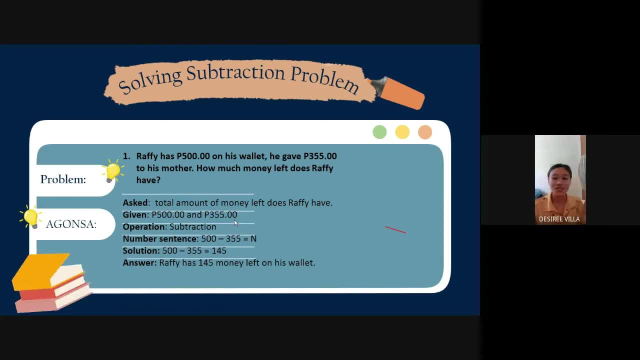 Alright, so thank you, Teacher Kay. Hello, good afternoon, students. Are you still there? Yes, teacher. 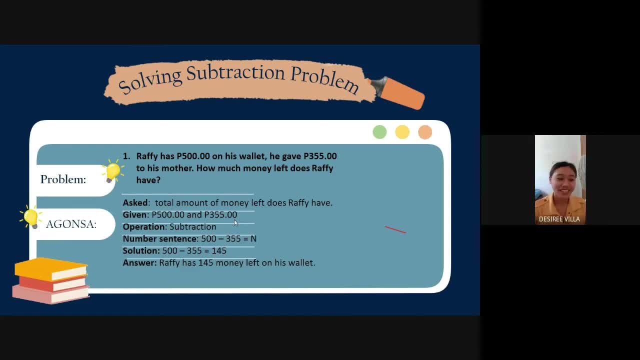 Alright, that's great. So, at this moment, let us now proceed to our next topic, which is, solving subtraction problem. 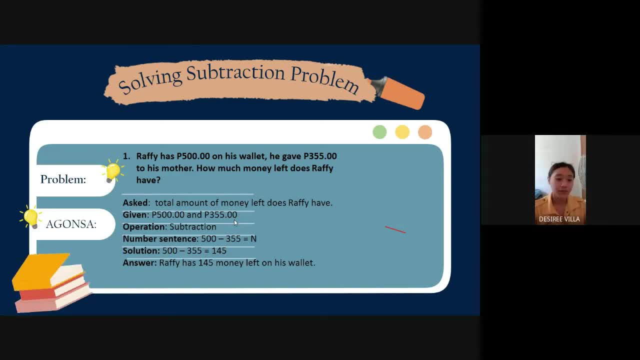 So, note that in this subtraction problem, we will also use, just like addition, we will also use agonza. But this time, the operation that we'll use is subtraction. So, 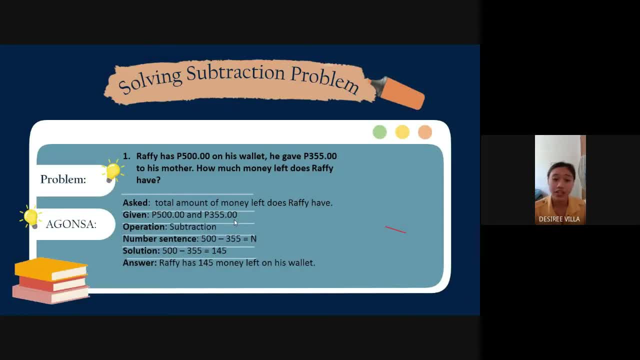 I have here another example, I mean, I have here example, yeah, subtraction. 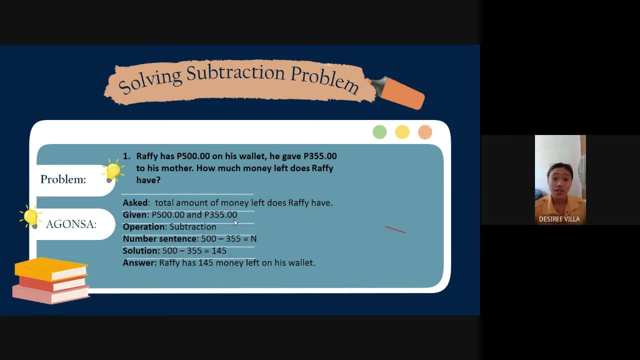 And note that agonza means that we have to give the what is asked, ok? 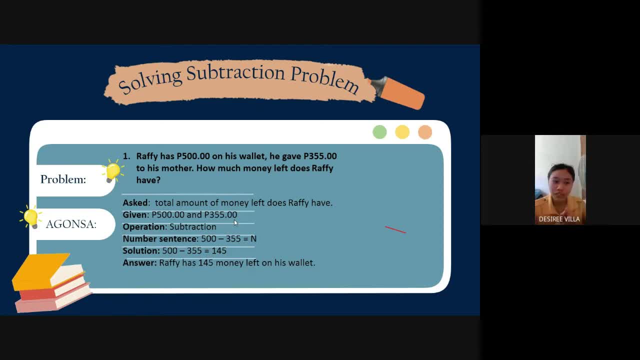 given um the operation that we will use the number sentence the solution and of course the answer so i have here an example of a number problem i mean red problem so may i ask somebody to read the problem on the screen who wants to volunteer 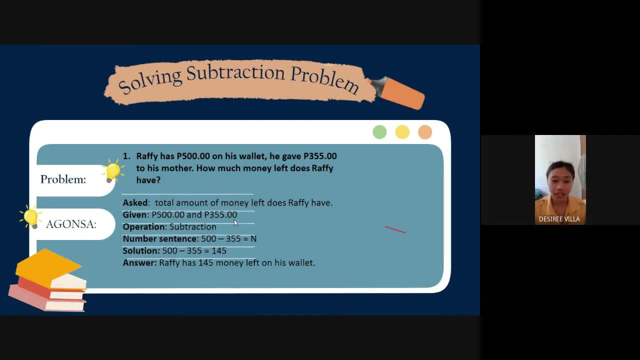 okay miss kimberly you you raised your uh you raised a hand so kindly read the problem on the screen 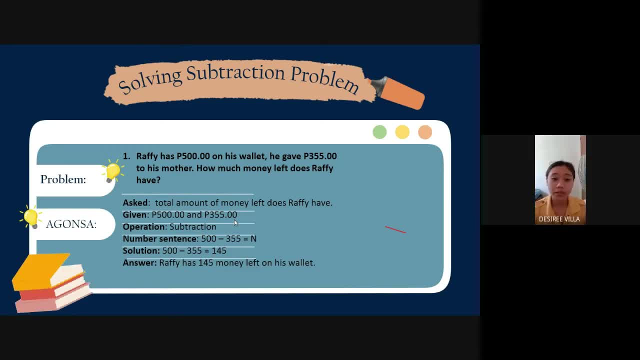 all right so thank you miss kimberly so the proper the problem here stays that see rafi cano 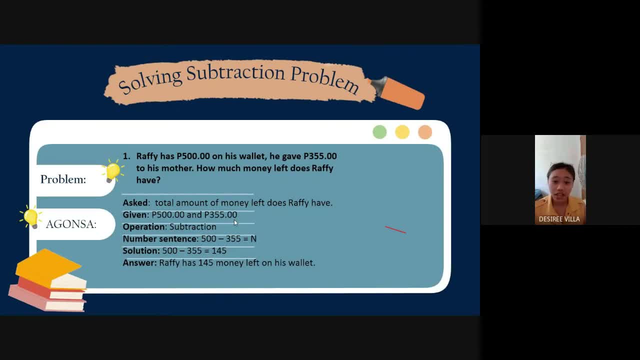 is 500 pesos and then he gave 355 pesos to his mother so the problem here is the answer is if rafi's wallet is already in line okay so line up so let's perform in agonza 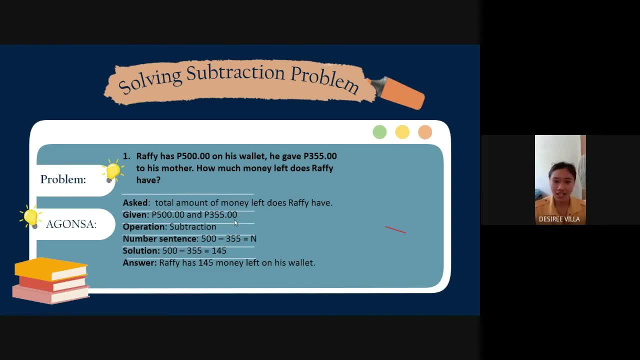 so first we have to give what is asked in the problem so the ask is what is the pereira box yes the total amount of money left does rafi have rafi have very good yes thank you 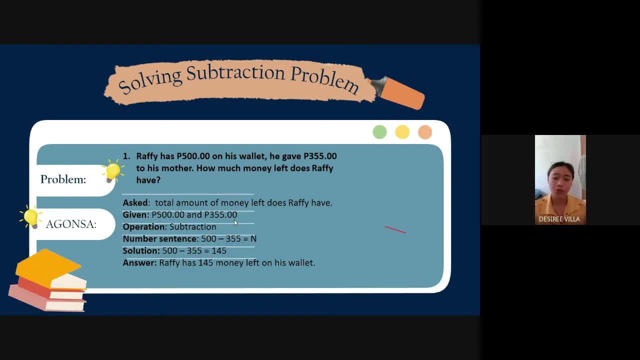 shane so next what is the given and the problem 500 pesos and 355 ms yes very good we have here the the given 500 pesos and 355. The 500 pesos is the original room of Raffy. And then we have 355 which is the room that was used by his mother. Alright, so what is the operation that we will use in this since the 500 pesos and 355? What is the operation that we will use? Alright, Mary Rose, you raised a hand. What is it? Subjection me. 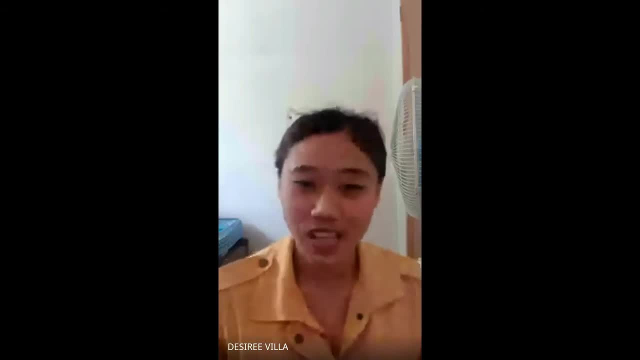 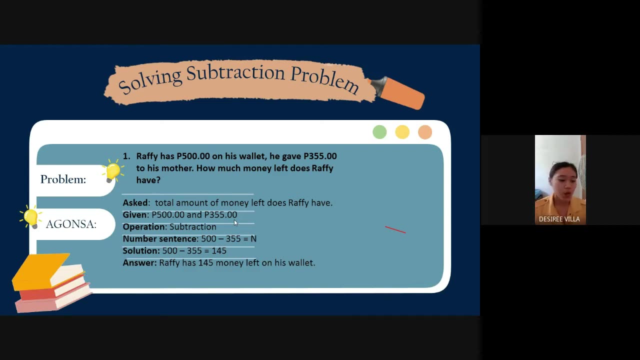 Very good. The operation that we will use in this problem is subtraction since 500 is 355. So how will you write 500 and 355 in a number sentence? Okay, Ms. Kimberly, you? 500 minus 300. 355 equals N. 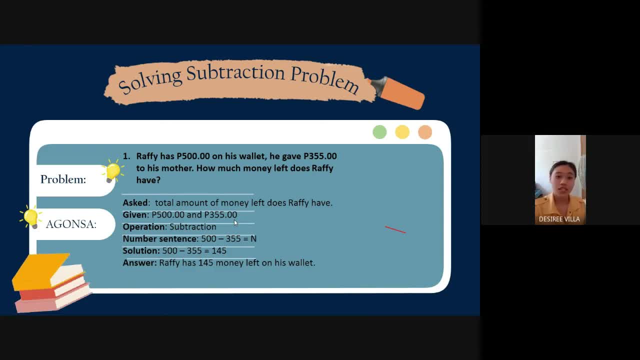 Alright, very good. So the number sentence will be 500 minus 355 is equal to N. We will write N since we haven't gotten the answer yet. 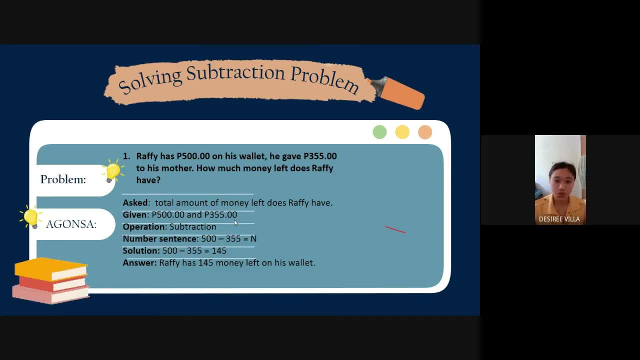 Okay, so that's why we will use the solution. 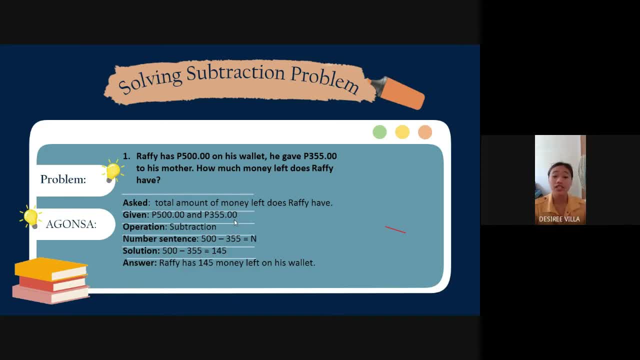 So the solution would be 500 minus 335. So we can subtract or subtract from one's place. 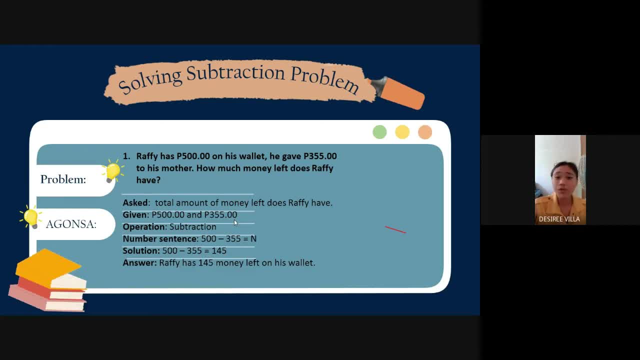 So we have here 355 and 500. So how many in one's place? Where is the one in 500? Zero means. Very good. Zero. 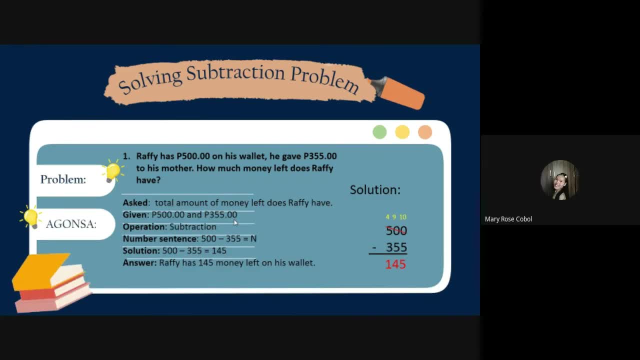 In the number of 355? Five. Very good, five. 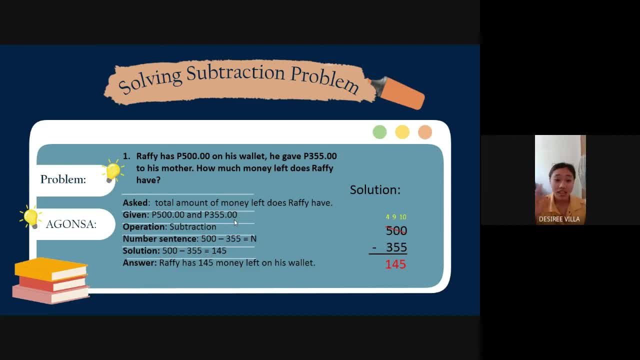 So zero minus five. five zero because zero is zero unless your value so that is why 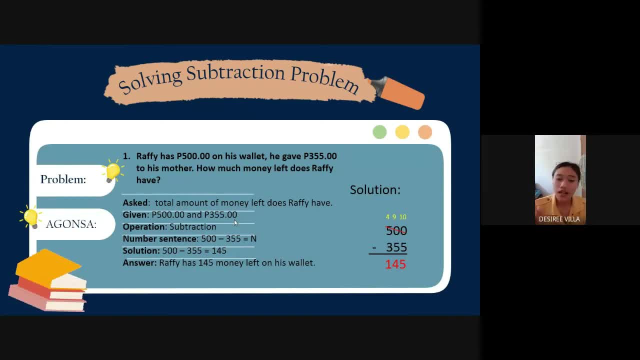 from the 10th place but since on 10th place the 500 is also zero hundreds place so 500 500 so i'm five my him on the nishang four so one is out of 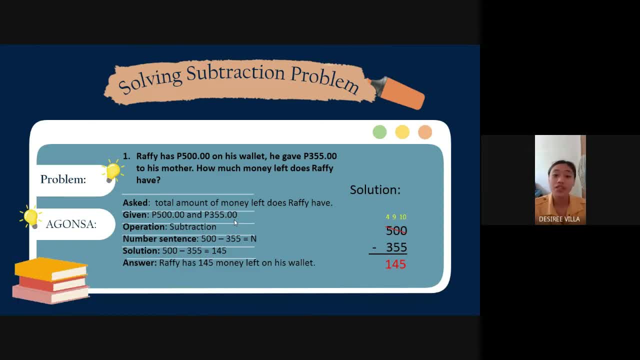 one's place will become ten so that maca subtract maca subtract mata so 10 minus five is equal to 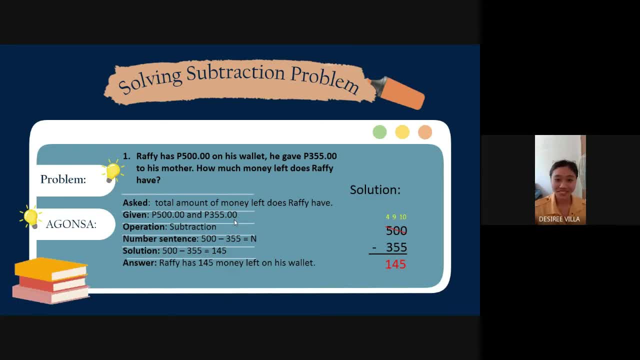 five yes very good ten minus five is equal to five so at least five below so 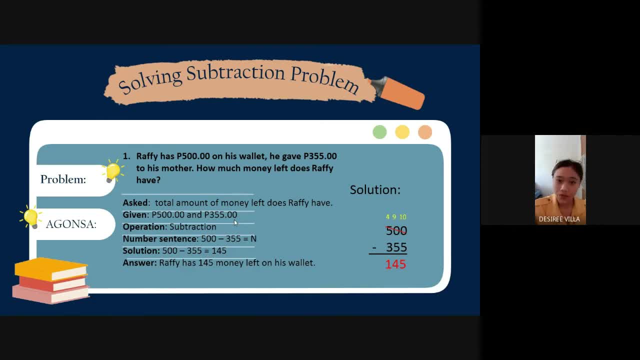 10th place nine minus five is equal to four so one of my nine money see happy cheering attend lucky on one's place so moment nine sha it's because me um from the one space okay so we bought four and then let's proceed to the hundreds place four minus three note that i'm four money 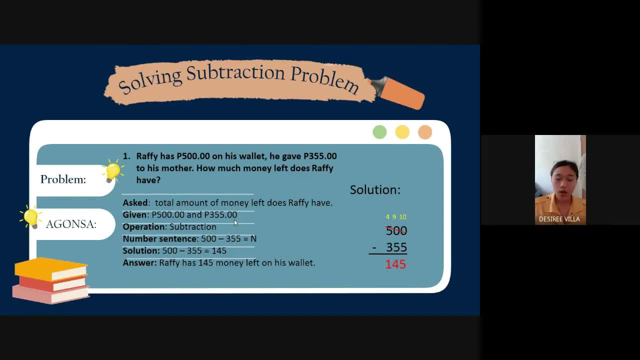 moshan four it's because me barota okay so four minus three is equal to 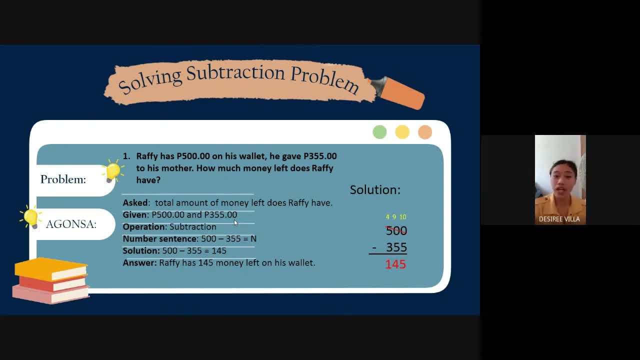 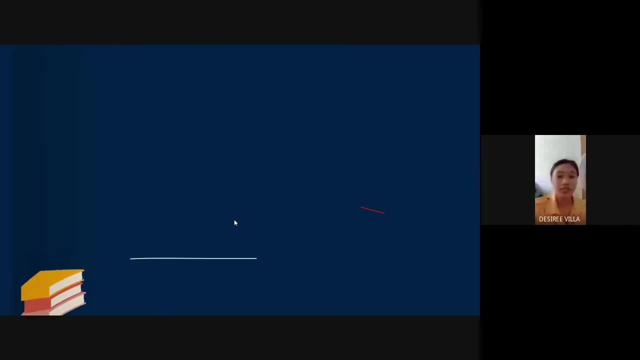 one one very good that's why we came up with an answer of 145. so let's go to the last letter of agatha which is a which means the answer so if we would answer this in a complete sentence it would be it would be raffi has 145.5 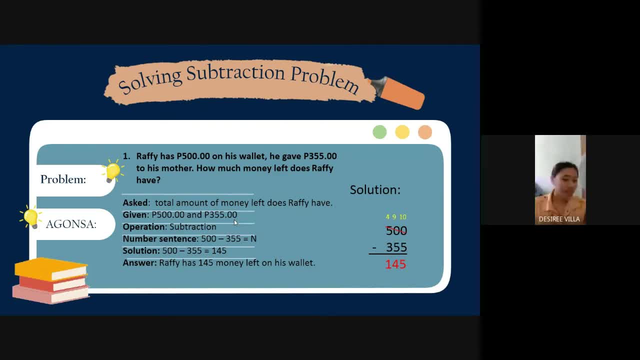 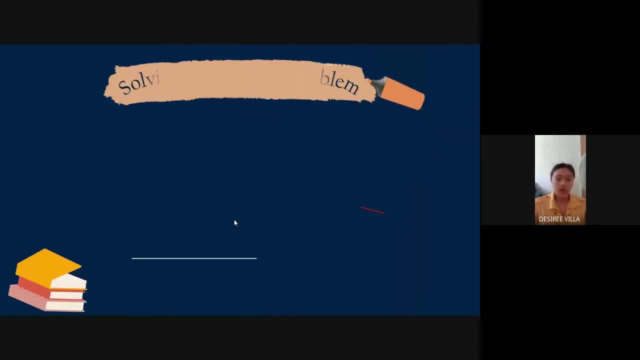 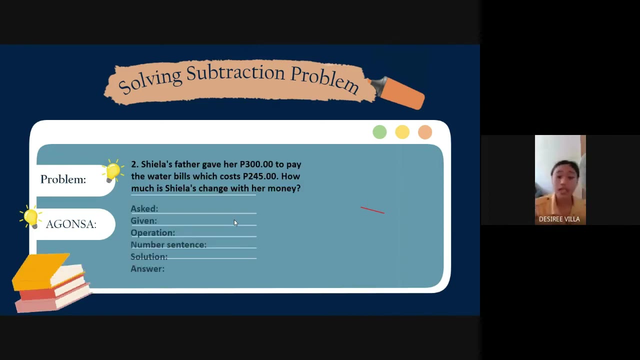 okay very good so next um i have here another word problem but this time okay so i will read the problem the problem for you and you will re you give me the agonza okay so 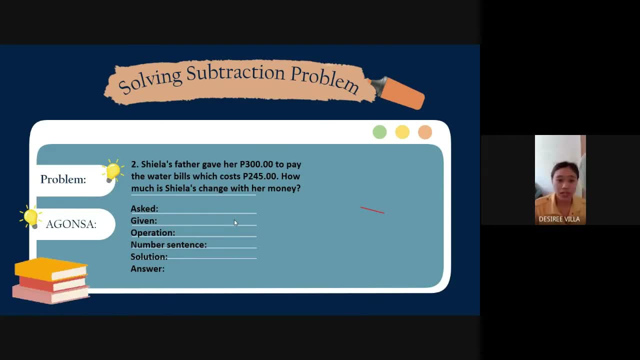 sheila's father gave her 300 pesos to pay the water bills which cost 245 pesos so how much is sheila's changed with her money all right so the problem here says that sheila konogi 300 pesos to pay say long water bills which costs 245 pesos right so the question is 300 right so grab it go subtraction or something okay 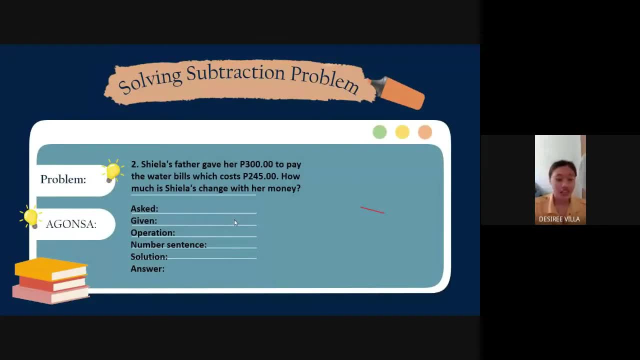 right so can i ask miss kimberly to give what is asked what is given the operation the number sentence the solution and the answer 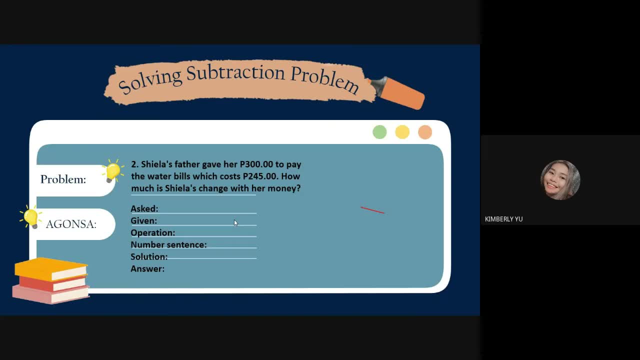 okay miss go on and ask me sky uh the number i how much is she let's change with her money then i'm given guy 300 passes and 245 passes the operation is subtraction and the number sentence is 300 pesos minus 245 equals n 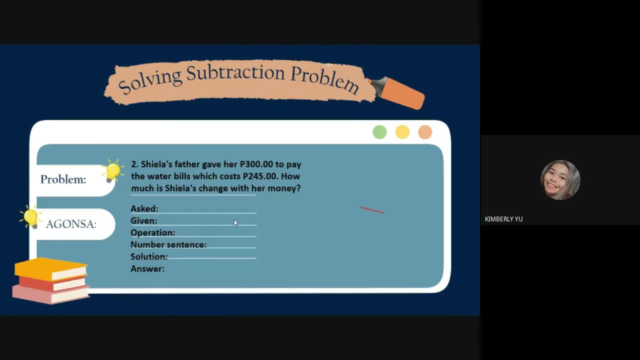 then our solution means 300 minus 245 passes equals 55 pieces and the answer is 55.25 pesos 245 pesos. 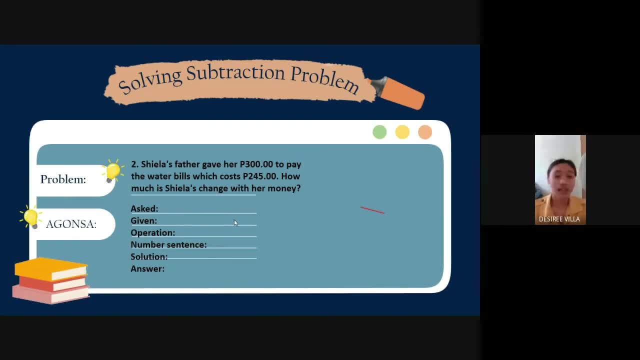 All right. So, thank you, Ms. Kimberly. Sakto ba ang gipang sulti ni Kimberly? Sakto ba ang ask? Ngayon gihatag? Ang given? All right. 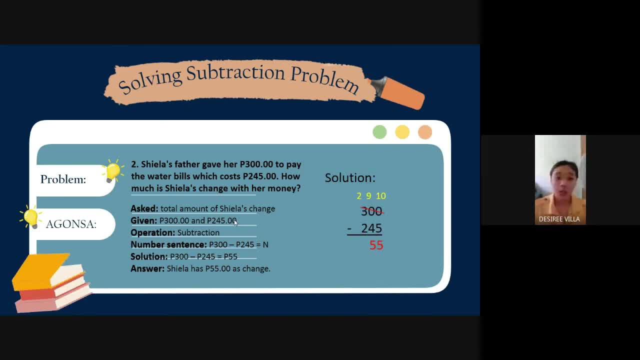 So, sakto. So, ang ask sa problem is the total amount of Sheila's change. Ka ang sukli daw ng gipang ayo. All right. 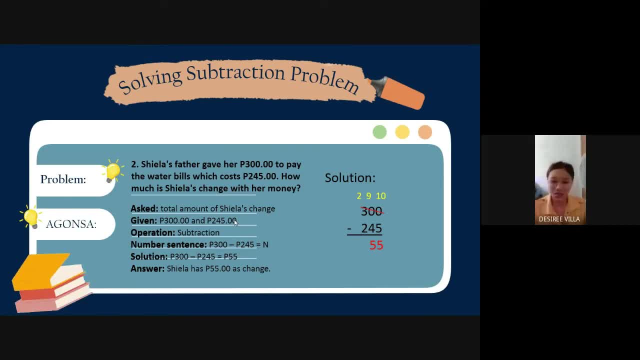 So, ang given. Ang 300 pesos and 245. Aksa mo ng 300. Aksa mo ng 300. 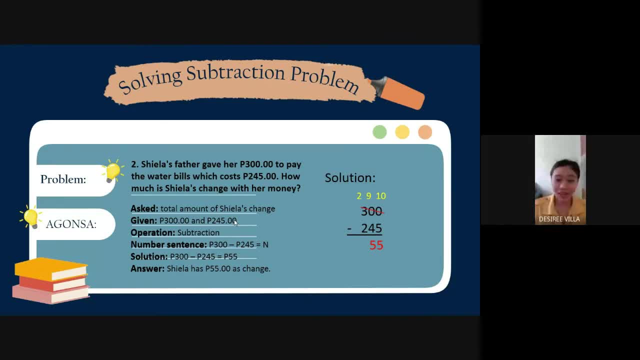 Ang 300 is ang gihatag sa iyahang papa. 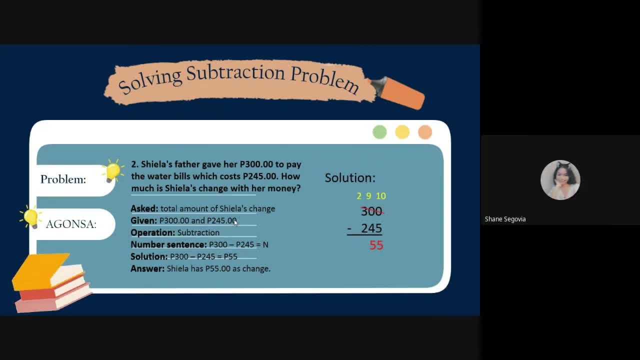 Ang buong kwarta. And the minuend. Very good, Shane. Thank you, Shane. 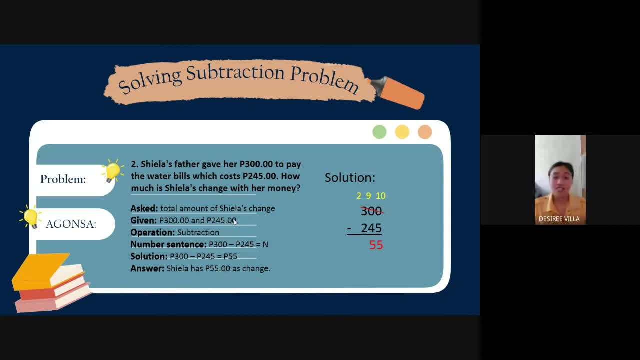 And the 245 is? This is the cost of the water bill. All right. So, nakasabot na ba? Nakasabot na ba, students? Any questions? No, Ms. Thank you. So, next. 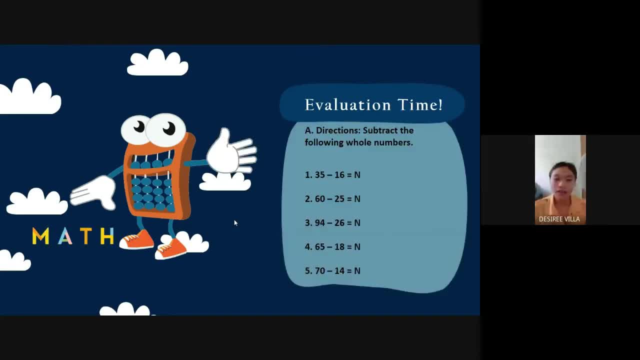 Okay, since naka-feel ko, naka-bantay ko na maayong nadyo kayo mga estudyante, ba? Bright, nakaayog akong mga estudyante. Okay, so, 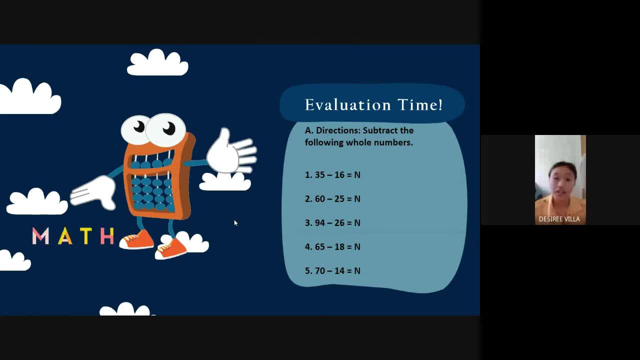 So, at this moment, I have prepared here five-item quiz para sa subjection. So, subtract the following whole numbers. So, the ring apart, I will call somebody to answer the questions, I mean, the items here, and then that somebody will call a friend to answer the next item. 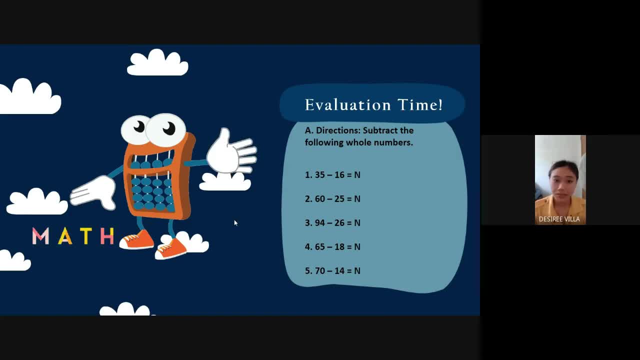 Okay? Kasabot na? Okay, Ms. Yes, Ms. Yes, Ms. Okay. Okay. That's good. That's good. 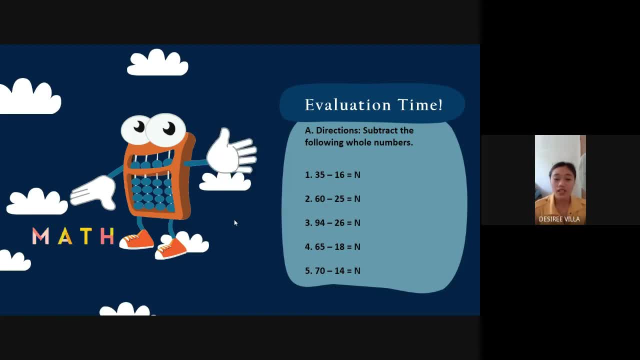 So, may I ask Ms. Mary Rose to answer number one, and then Mary Rose will call a friend to answer number two. 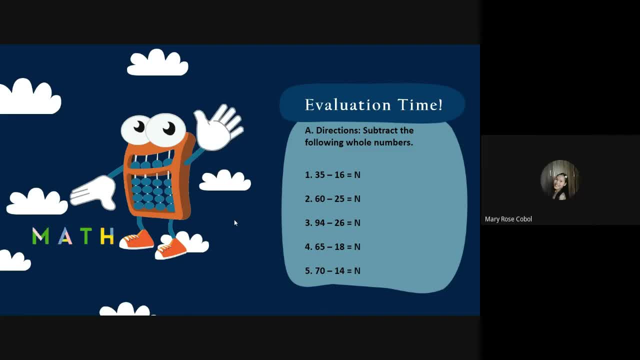 Thirty-five minus sixteen equals nineteen, Ms. Very good. 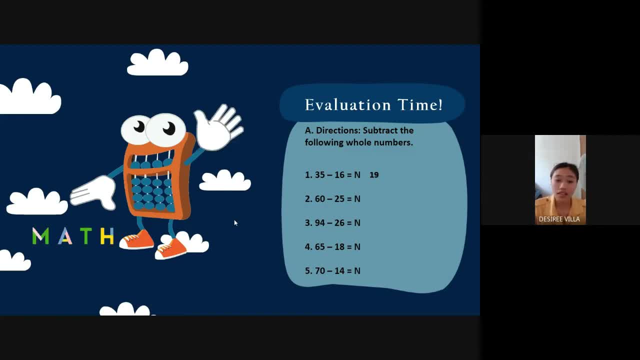 How did she get nineteen? Ba? Ba? Ba. Ba. 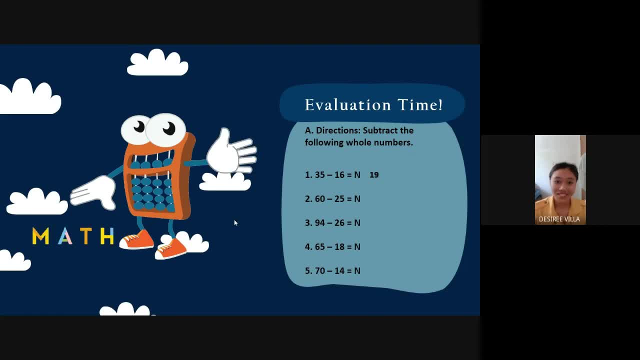 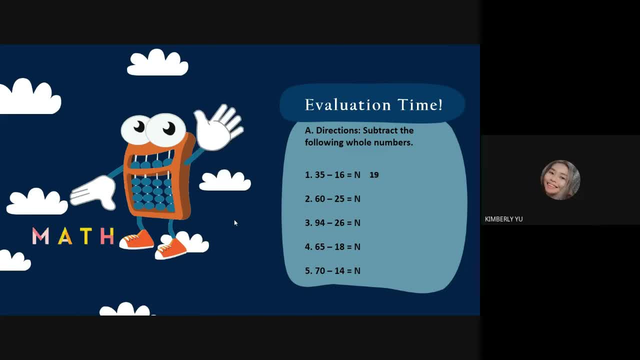 Yes, Ms. Sixty minus twenty-five equals thirty-five. Thirty-five. 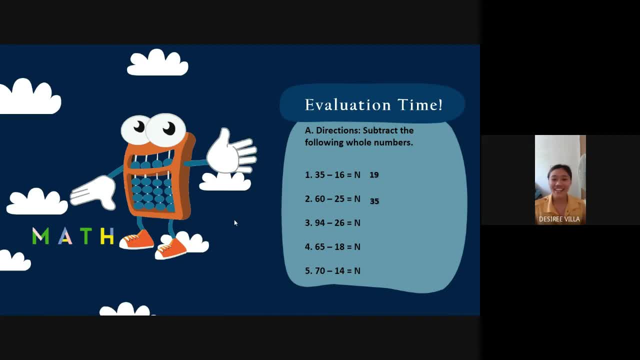 Let's check. Alright! So, sixty minus twenty-five equals thirty-five. So, 60 minus 25 is 35. Very good. 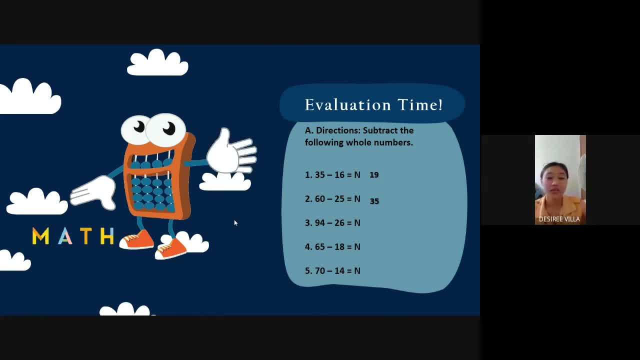 Kabaytas ako mga estudyante. Uy, wala na may padugay-dugay. Next. Number three. 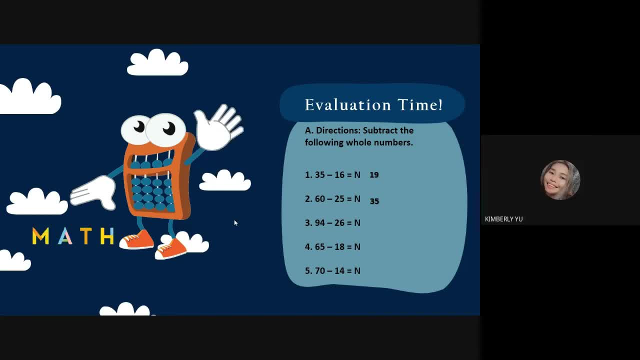 Kinsayong paansiran, Miss Kimberly. Si Jasper, Miss. Jasper. 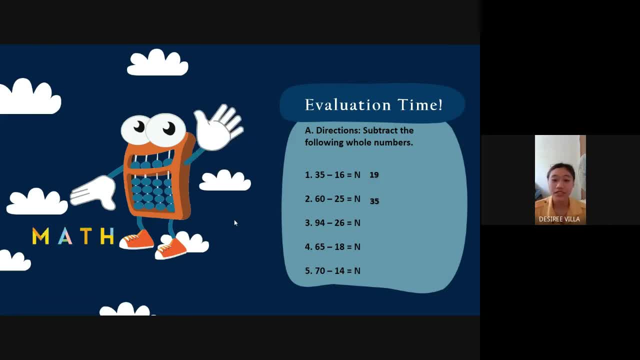 Please turn on your microphone. Please unmute yourself. 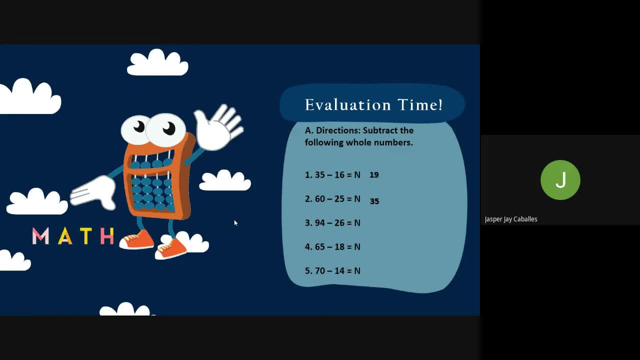 Okay, Jasper. 24 minus 26 equals 68, Miss. Very good. Halakabrayt. Uy, makabilib. 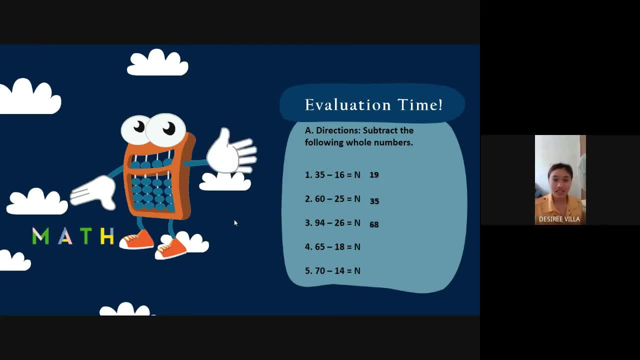 Okay, so 94 minus 26 is 68. So, Mr. Jasper, kinsayong paansiran number four. So, same. Okay, Miss Jane. 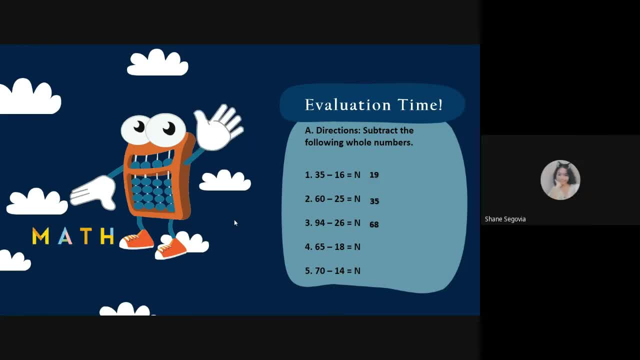 65 minus 18 equals 47, Miss. 47. Very good. Very good, Jane. 65 minus 18 is equal to 47. So, last number, five. Who wants to answer number five? Voluntary na lang. I'd like to. Okay. Okay. Me, Miss. Go on. 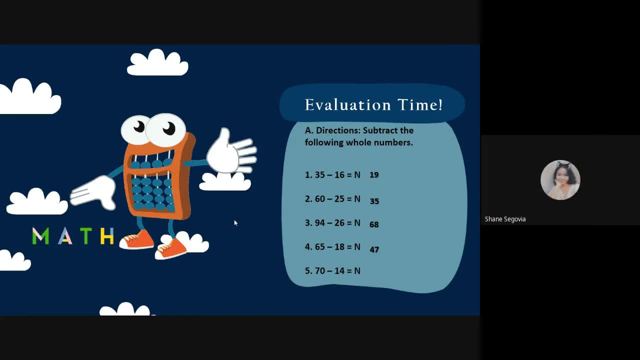 70 minus 14 equals 56, Miss. 56? No. Let's check. All right. 56. Perfect. Ka-broitso ko mga students. 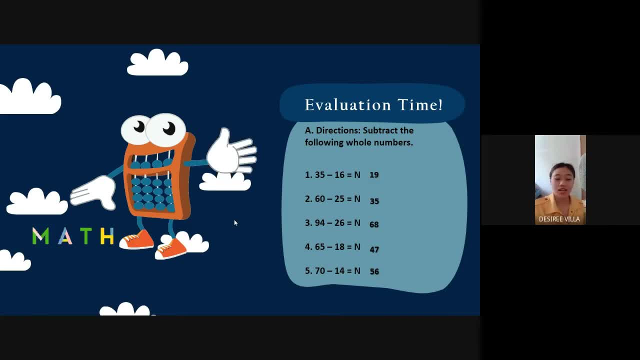 70 minus 14 is equal to 56. So, give. 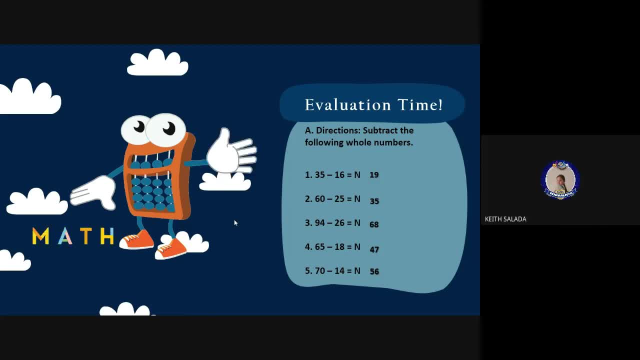 Pak-pak. Ka-broit na kayo mga students. All right. I'm so proud of you. So, next. 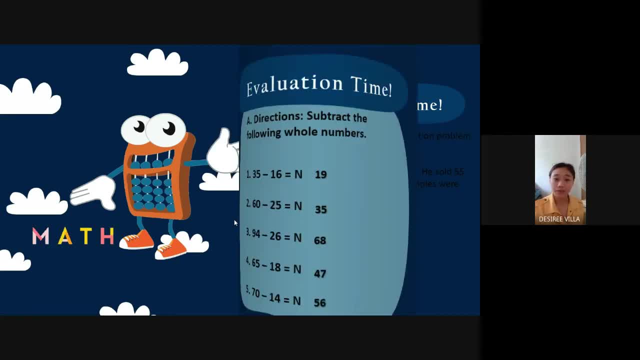 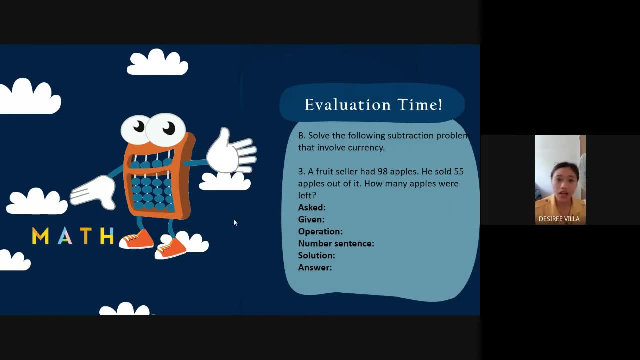 For the letter B evaluation, this is a number problem. So, who wants to volunteer to give the gansa of this problem? Anyone? Anyone. So, let's see. Let's see. We're gonna go through this. Okay. 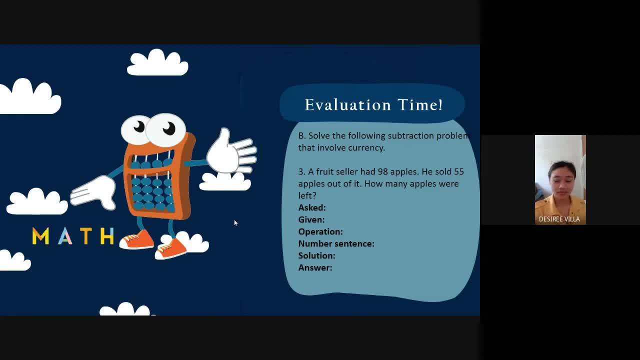 So, let me just call on Miss Kimberly Yu to answer this. Okay. Well. Yeah, Gonzo. 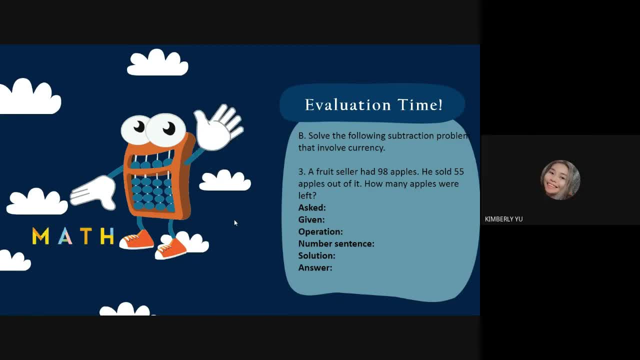 Shane likes to answer, Maze. Shane wants to answer. Shane wants to answer? Okay, go, Shane! 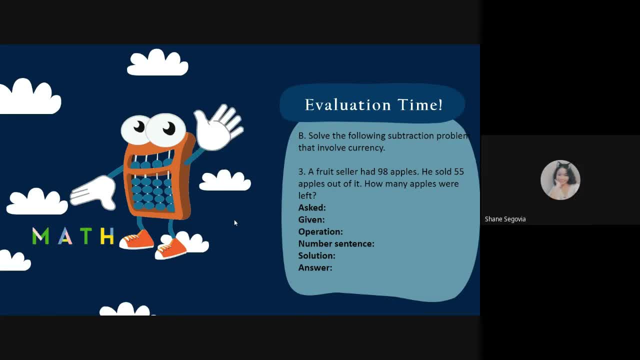 My screen is kind of blurry right now, Maze, because of maybe the internet connection, but please guide me, Maze, if ever I couldn't read, Maze. 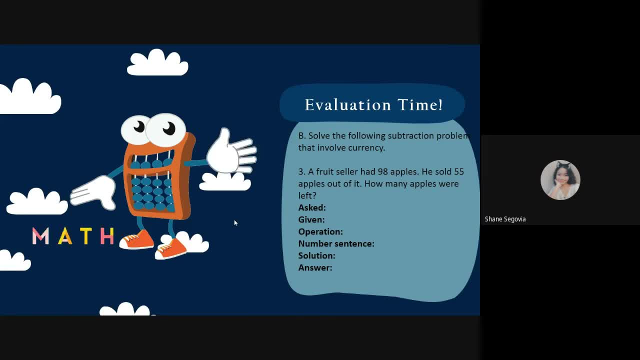 So, a fruit seller had 98 apples. He sold 55 apples out of it. How many apples were left? Okay, that's the problem. 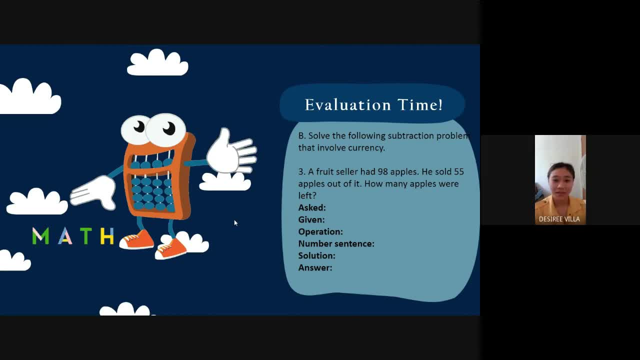 I'm gonna answer the Agonza, Maze. Yes. Go, Shane! Okay. 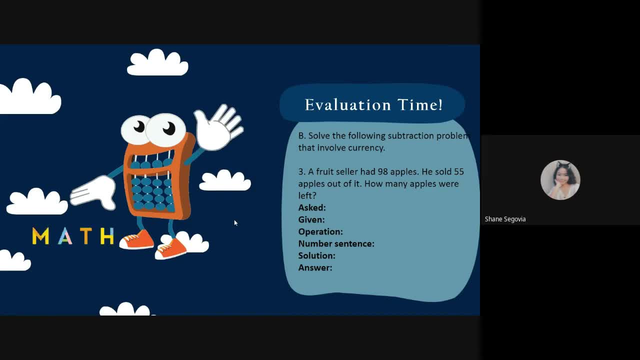 So, what is asked there is the total apples left. 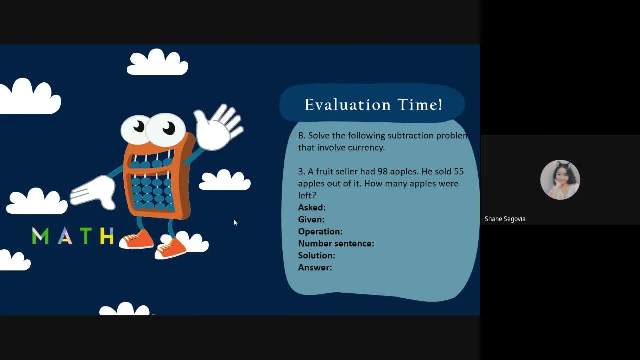 And the given is 98 apples and 55 apples. 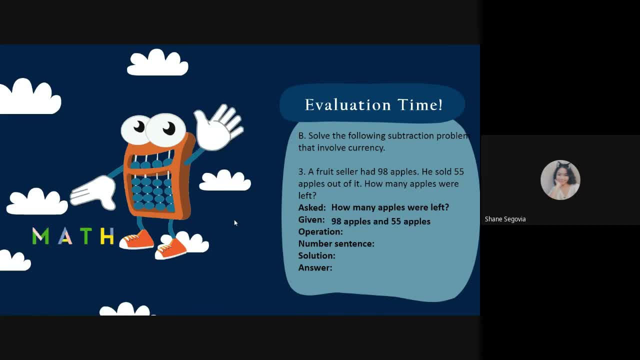 The operation used is subtraction. 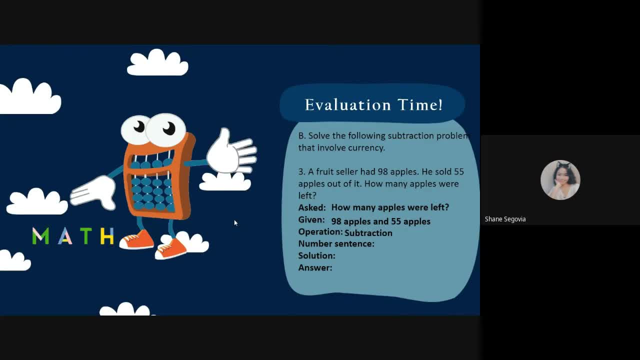 The number sentence there is 98 minus 55 equals n. 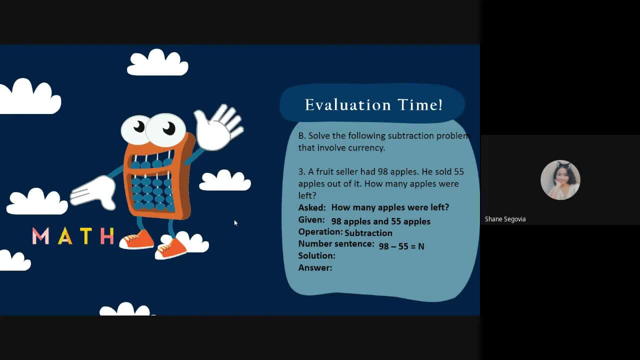 And the solution is 98 minus 5 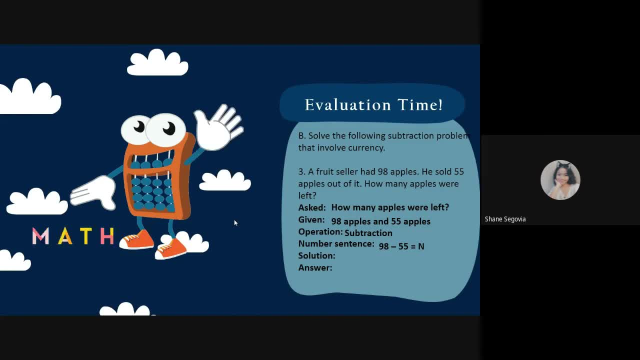 are 43 apples left. 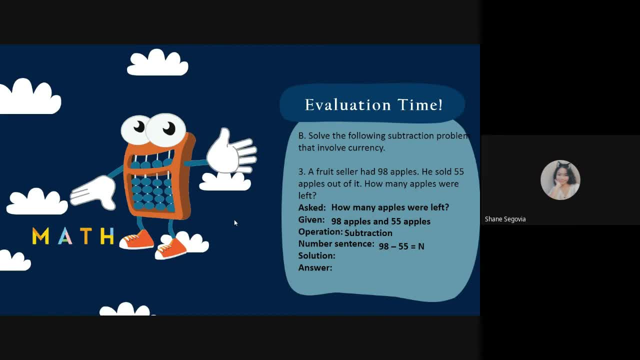 Let's check Shane's answer. 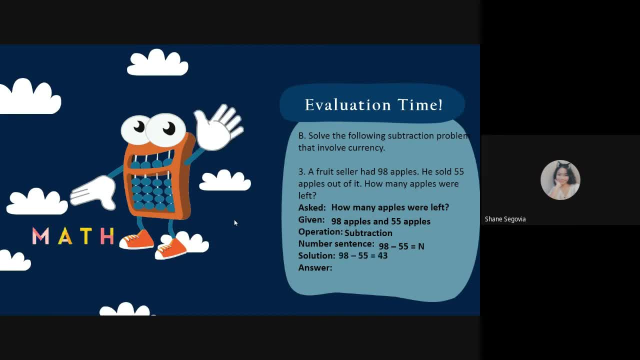 Okay, the ask is how many apples were left. And the given is 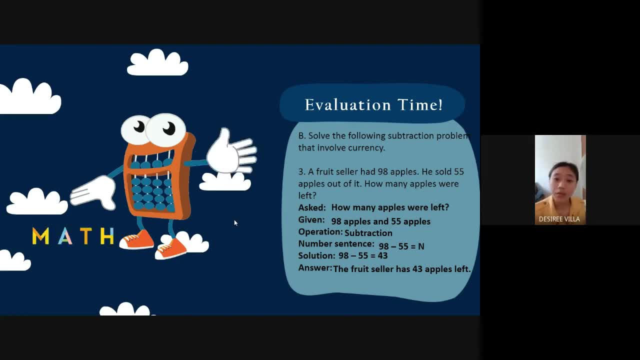 how many apples were left. 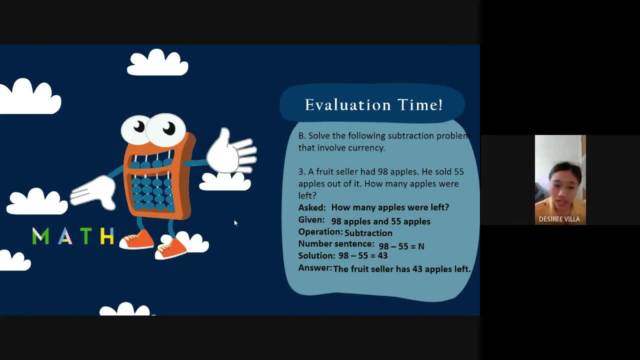 And the given is 98 apples and 55 apples. 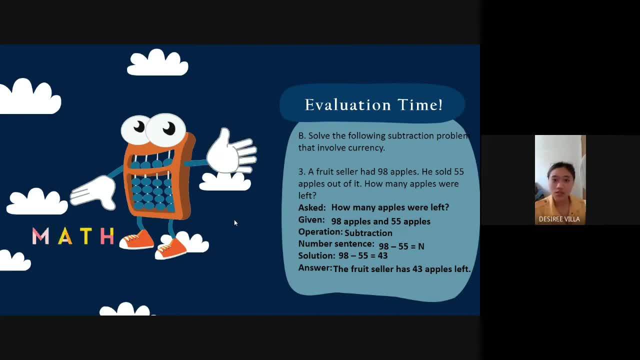 So, the operation that we will use is subtraction. Shane is correct. So, the number sentence would be 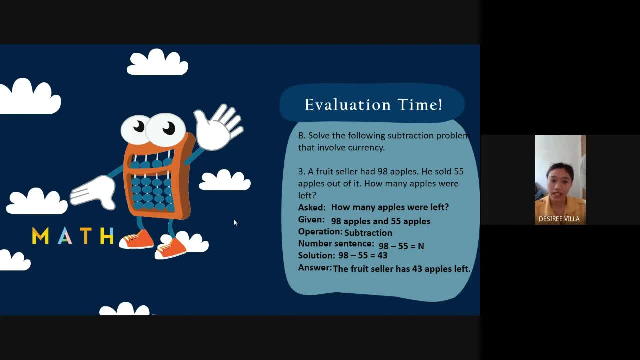 98 minus 55 is equal to n. And the solution 98 minus 55 is 43. 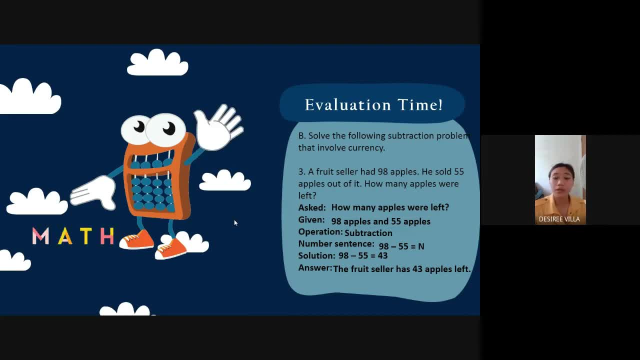 Okay, and the answer would be and the answer in a complete sentence would be the fruit seller has 43 apples left. Very good, Shane. Can you give Shane a wall clap? 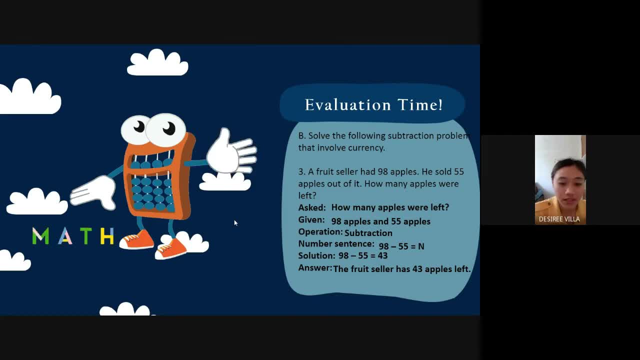 Okay, unmute yourselves. 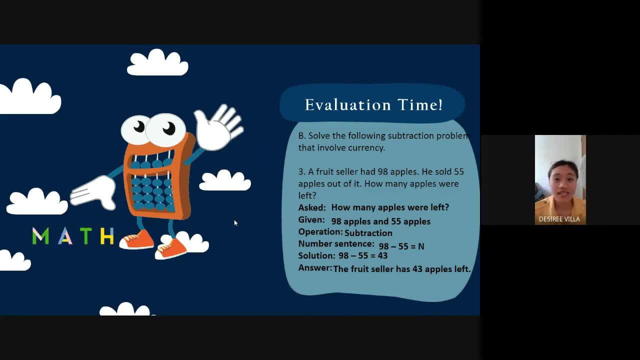 Okay, very good. So, next. 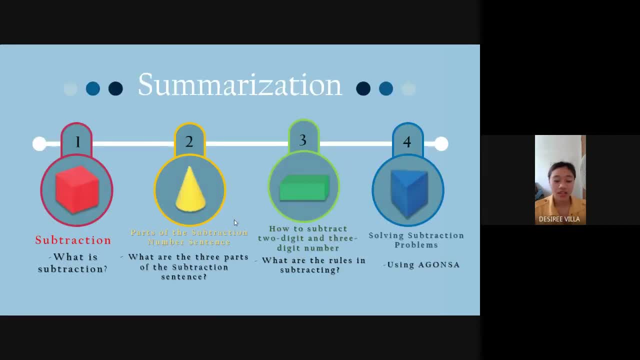 Next, though. To summarize our topic for today, I have prepared here some questions for you to recall our topic for today discussed with Teacher K and Nako. So, what is our topic for today again? Okay, Mr. Jasper. 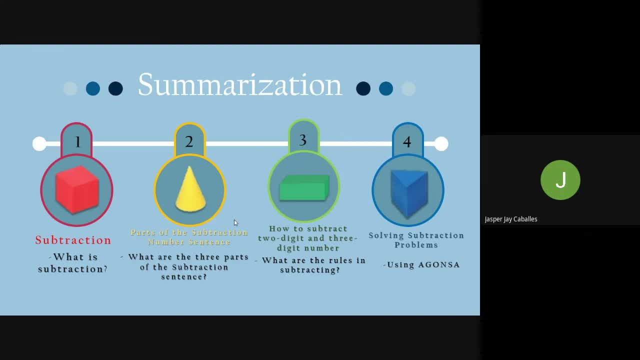 It's all about subtraction myth. Very good. Our topic for today is about subtraction. 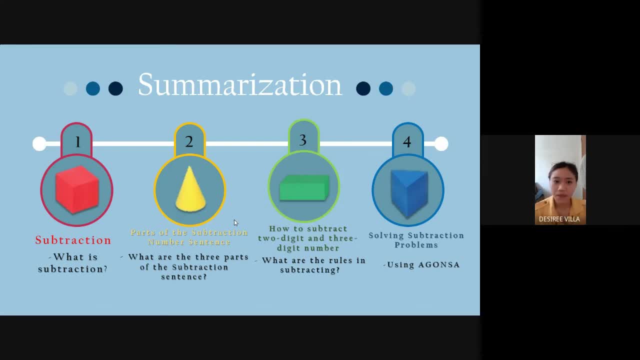 And so, what is subtraction? What is subtraction? What is subtraction? Miss Mary Rose, you raised a hand. What is subtraction? 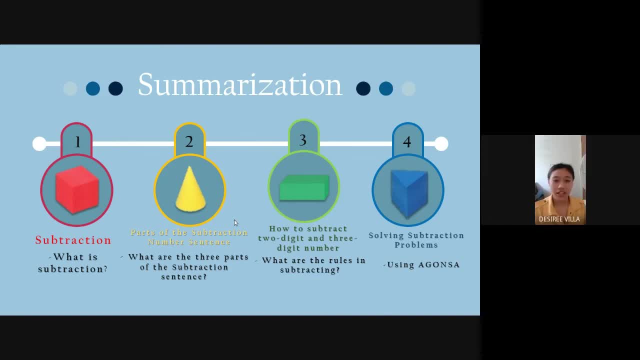 What is subtraction? Very good. 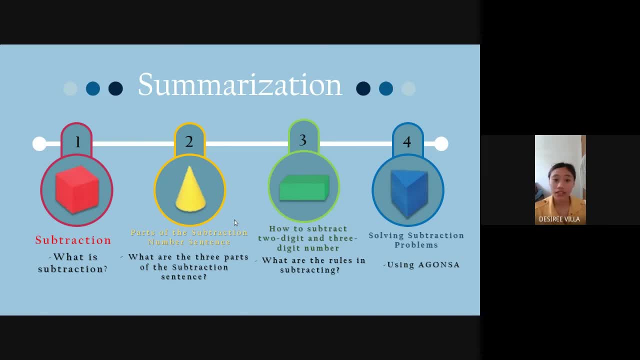 What is the number? What is the number? Number set. So, next is parts of the 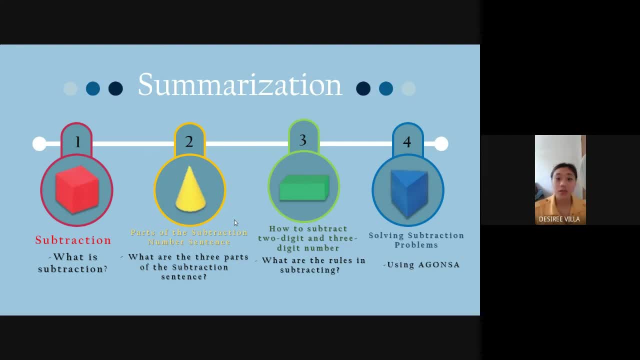 Wait. Parts of the subtraction 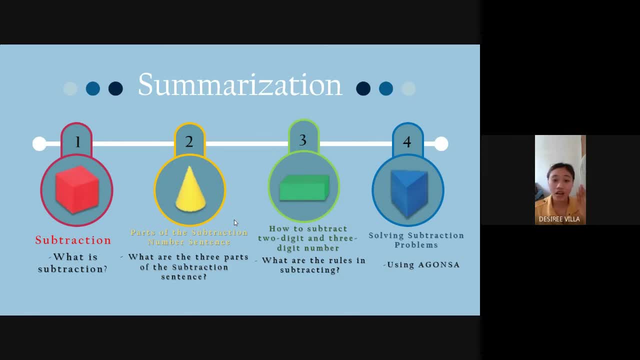 number sentence. So, what are the three parts of the subtraction sentence? Yes, Miss Shane Kimberly? 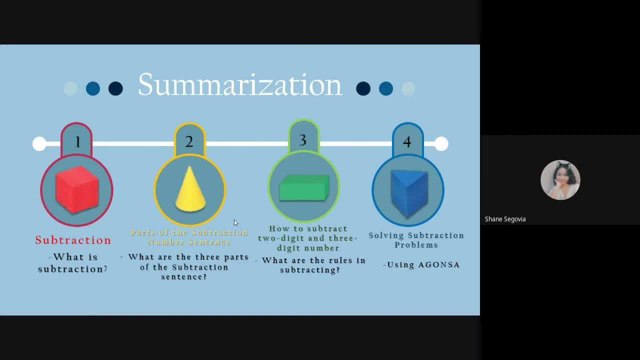 The three parts of the subtraction sentence includes the minuend, the subtrahend, and of course, the 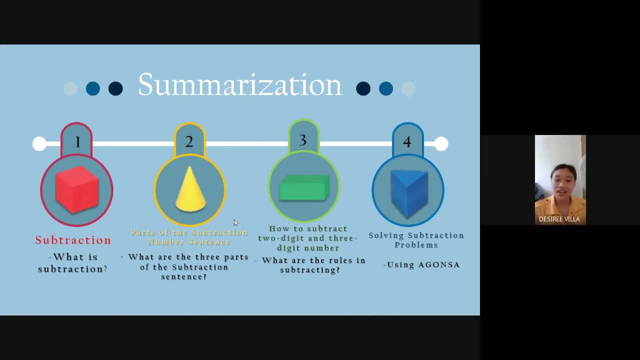 difference mace. Yes, very good, Shane. Thank you for that. 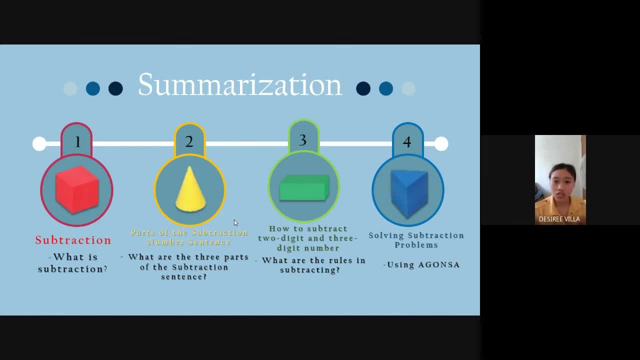 And next, how to subtract two-digit and three-digit number? Where do we use this? I mean, yes. What are the rules? 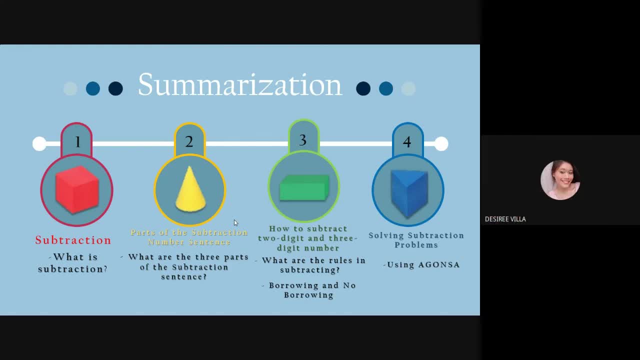 Yes? Yes? Yes? 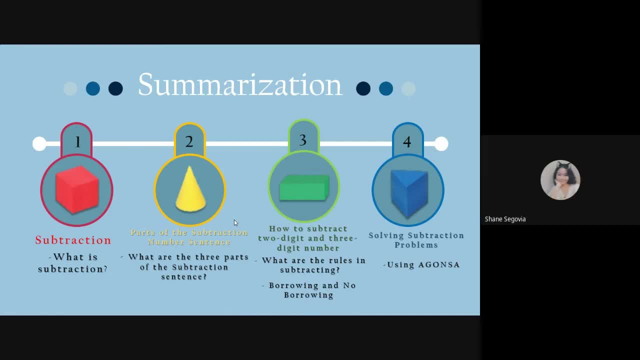 What does it mean? Borrowing and 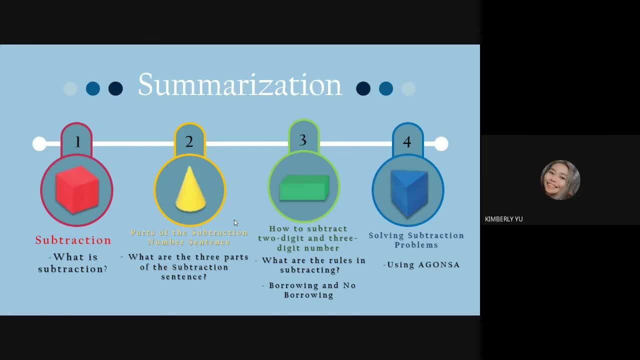 Borrowing and Yes, borrowing and 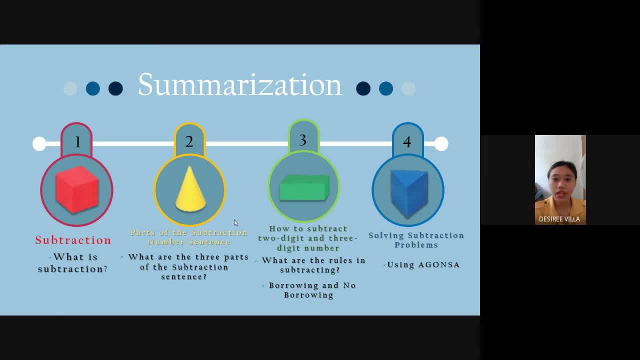 Very good. It is borrowing and no borrowing. 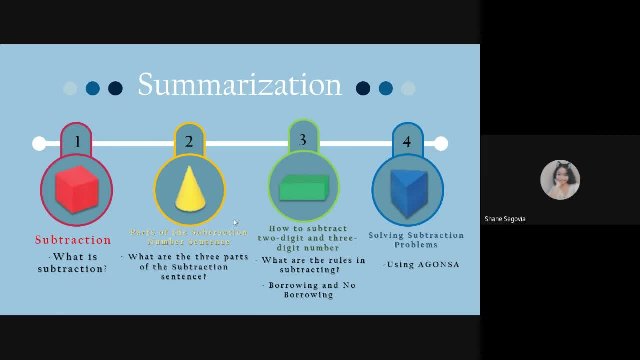 So, in solving Borrowing and 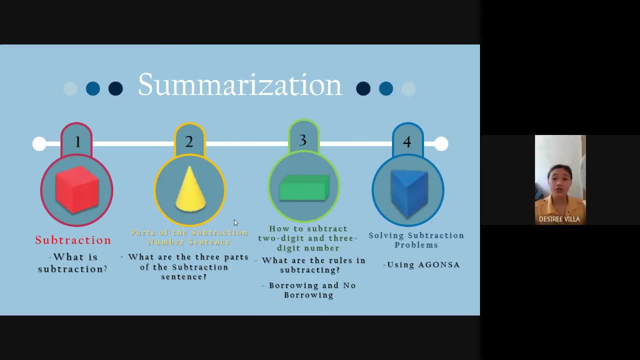 no borrowing. Yes, very good. Thank you, Shane. 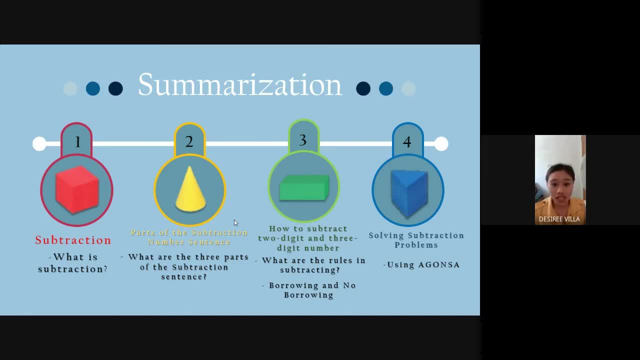 So, in solving subtraction problems, what process do we use? 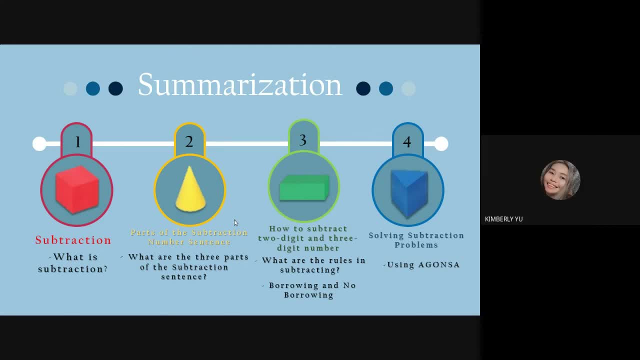 We're using Agonza, Miss. Very good, Kimberly. 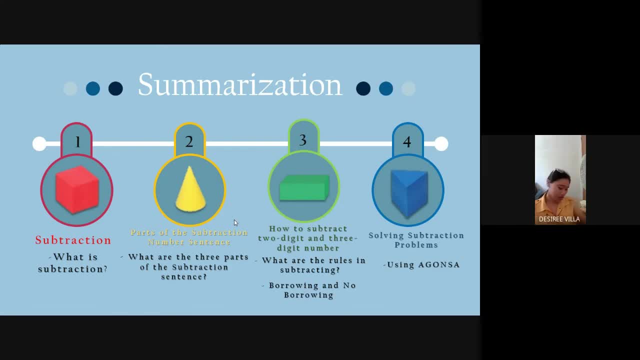 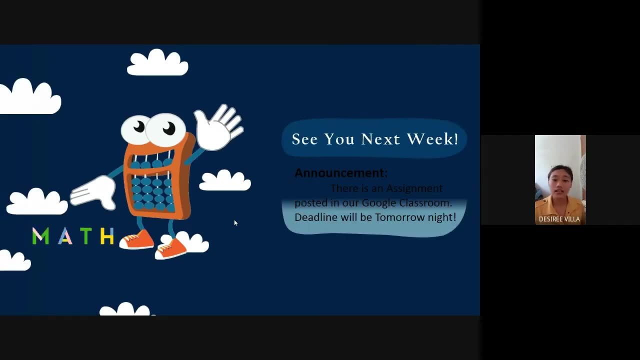 We are using Agonza. So, next, I have posted I have posted items on our Google Classroom and I want you to answer that honestly. 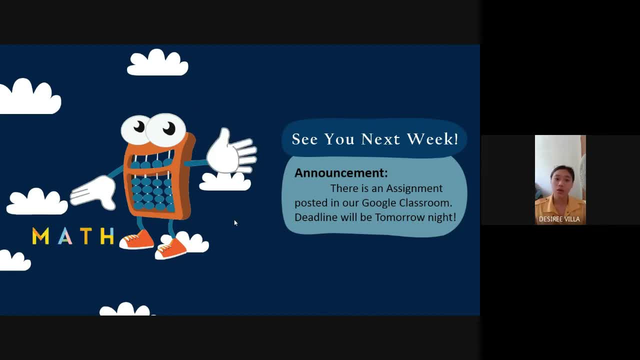 It is our assignment. It is posted in our Google Classroom. I want you to answer it honestly and I hope that you will pass it before or on the deadline. I don't accept late. 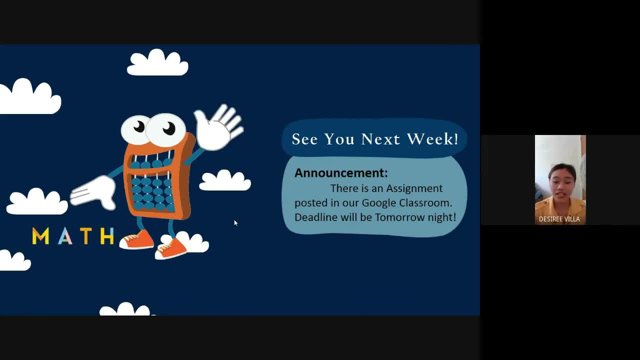 Okay? Do you understand, students? 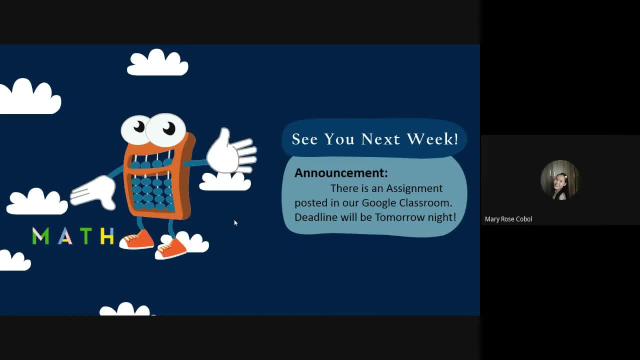 Do you understand? Yes, Miss.